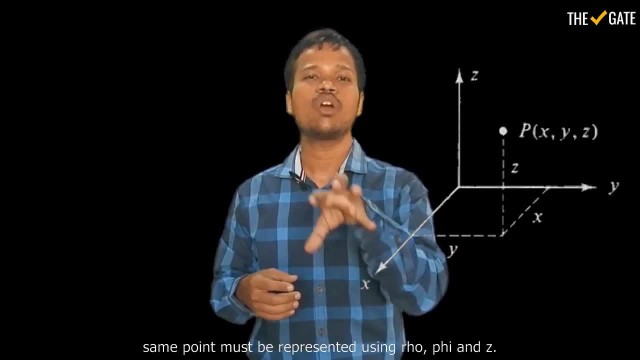 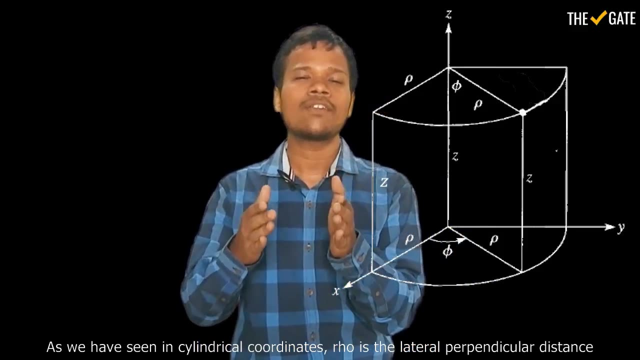 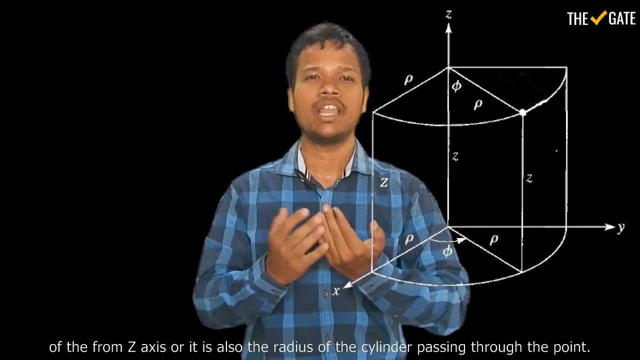 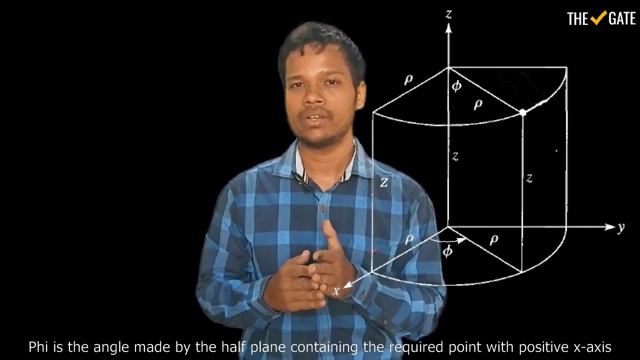 then the same point must be represented using rho, phi and z And, as we have seen in cylindrical coordinates, rho is the lateral perpendicular distance of the point from z axis, or it is also the radius of the cylinder passing through the point. Phi is the angle made by the half plane containing the required point, with positive x axis. 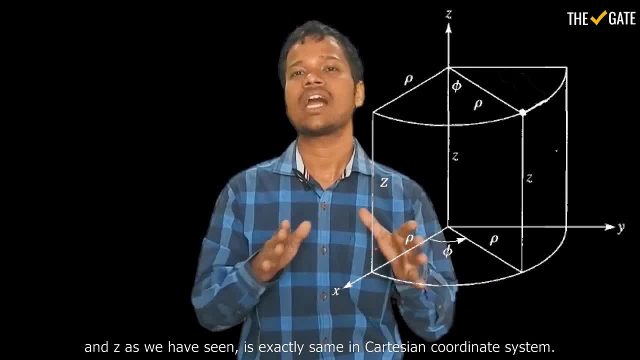 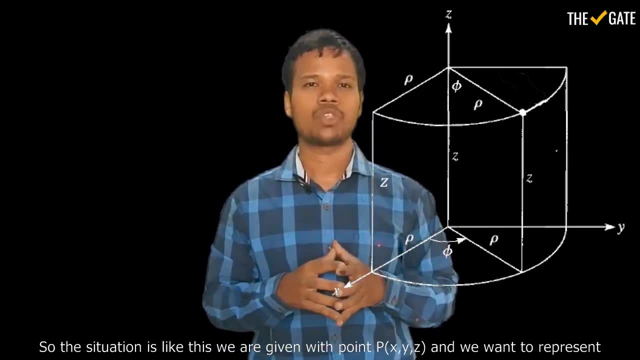 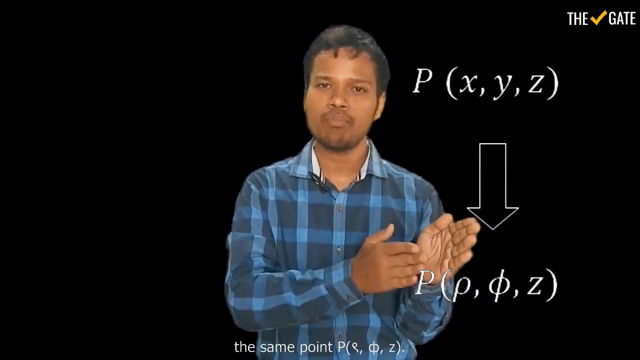 And z, as we have seen, is exactly same in Cartesian coordinate system. It is the perpendicular distance from x y plane. So the situation is like this: We are given with point P, x, y and z And we want to represent the same point, P rho. 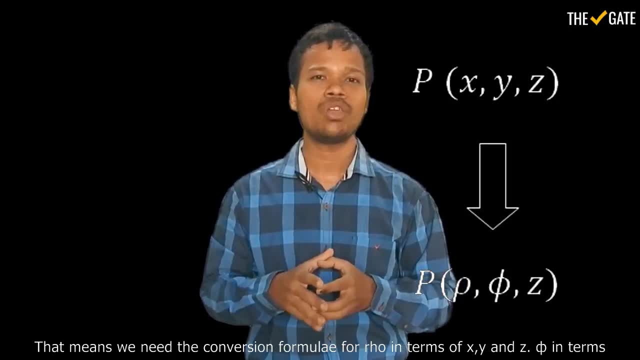 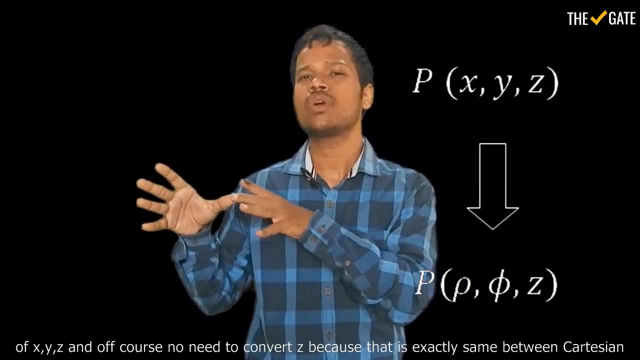 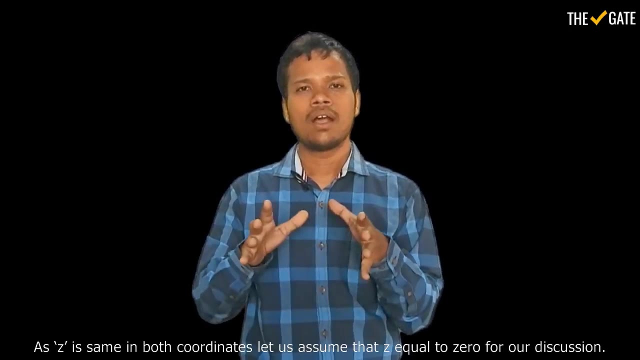 phi z. That means we need the conversion formula for rho in terms of x, y and z phi in terms of x, y and z. And of course no need to convert z, because z is same between Cartesian and in cylindrical coordinates. As z is same in both coordinates. let us assume z equal to zero for our description. 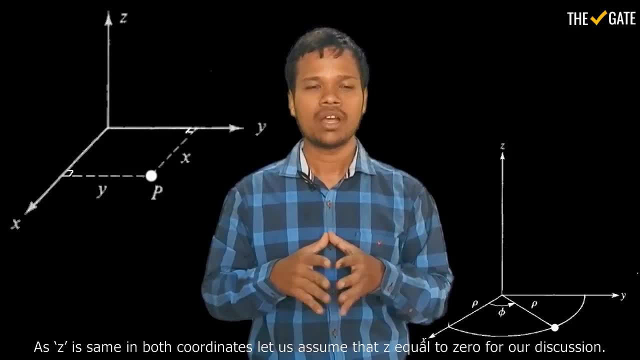 And we would use the remembers formula for coefficient y, з, what we guess is 0. so z is our second previous kingdom and z is our second Ты. the relationship over this is our description. that means, let us assume that our point is present on XY plane. so 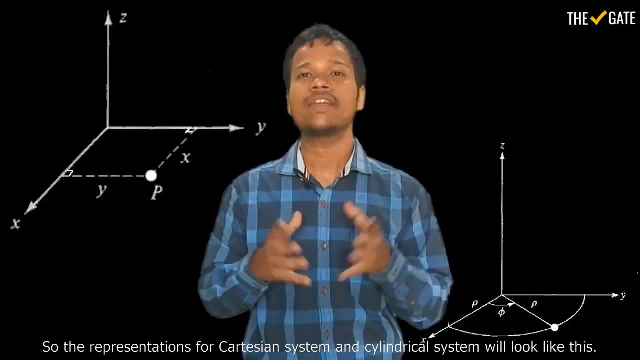 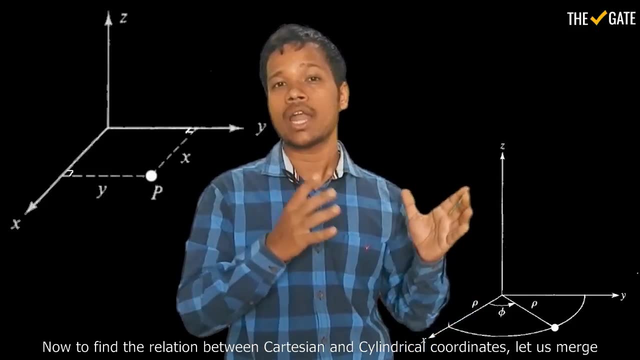 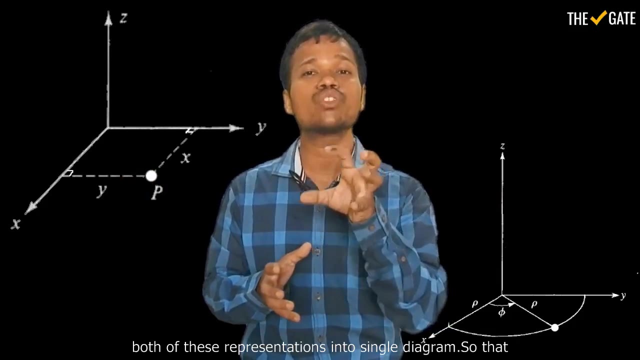 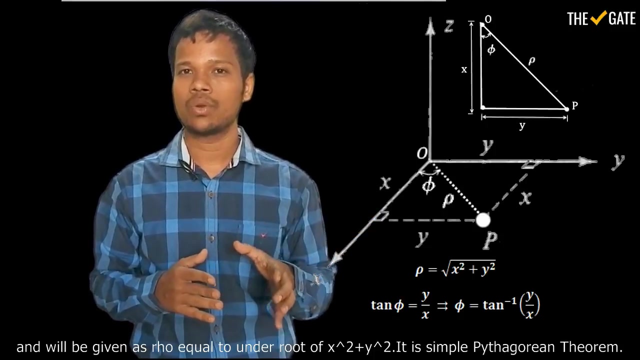 the representations for Cartesian system and cylindrical system will look like this. now to find the relation between Cartesian and cylindrical coordinates, let us merge both of these representations into single diagram. so you can clearly see in the diagram in the right angle triangle who is the hypotenuse, and it will be given as rho equal to under root of X square plus Y. 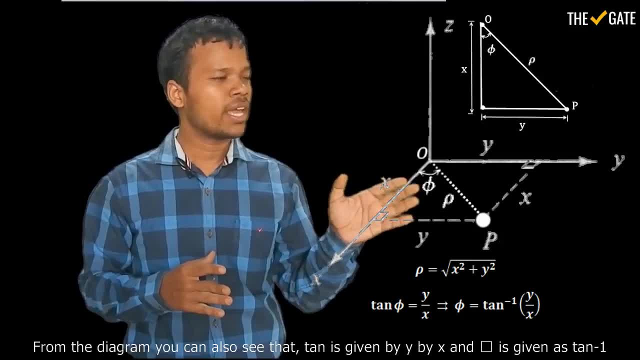 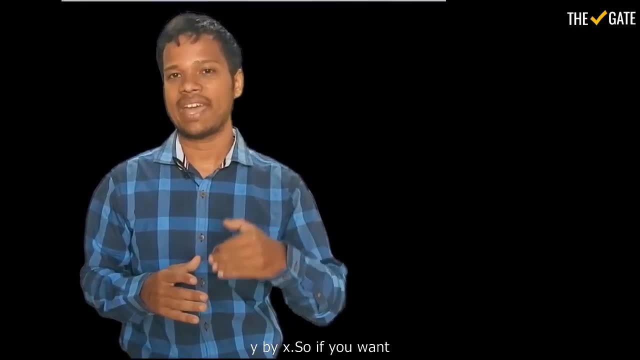 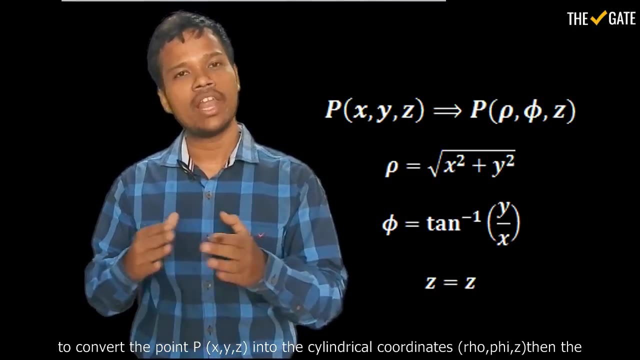 square. it is simple Pythagorean theorem. from the diagram you can also see that tan Phi equal to I by X. so Phi will be given as tan inverse Y by X. so if we want to convert the point P, XYZ into cylindrical coordinates, rho, Phi and Z. 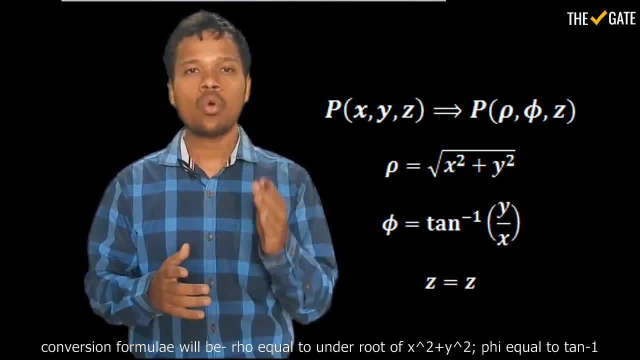 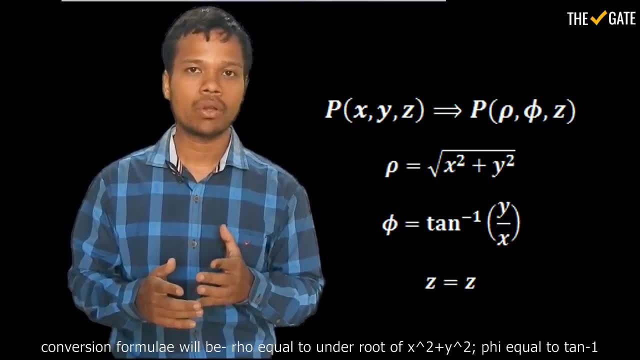 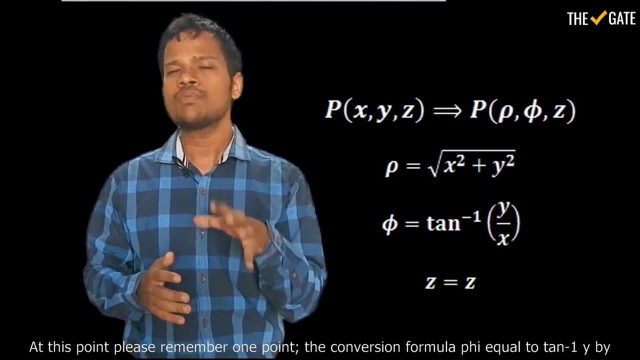 then the conversion formula will be rho equal to to under root of x square plus y square. phi equal to tan. inverse y by x and z. of course z will be the same, z equal to z. at this point, please remember one point: the conversion formula, phi equal to tan. 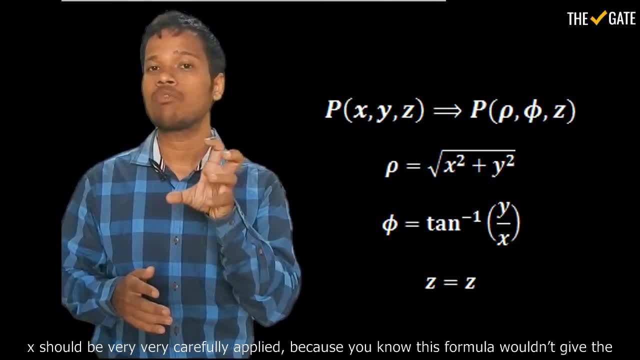 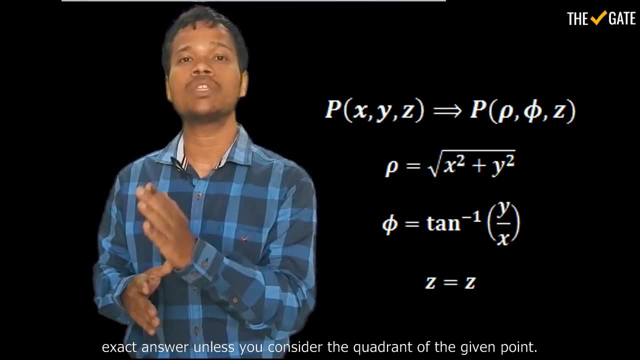 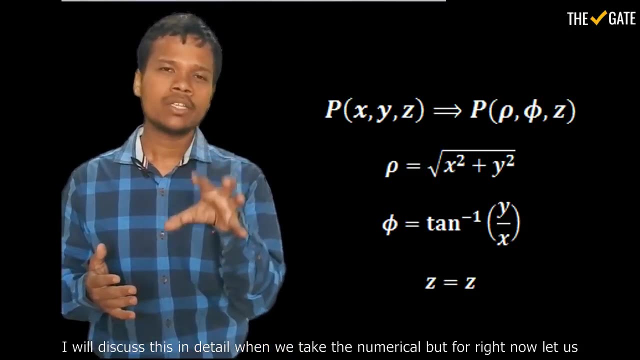 inverse y by x should be very, very carefully applied because you know this formula wouldn't give you the exact answer unless you consider the quadrant of the given point. so this formula is slightly modified for different quadrants of the point. i will discuss this in detail when we 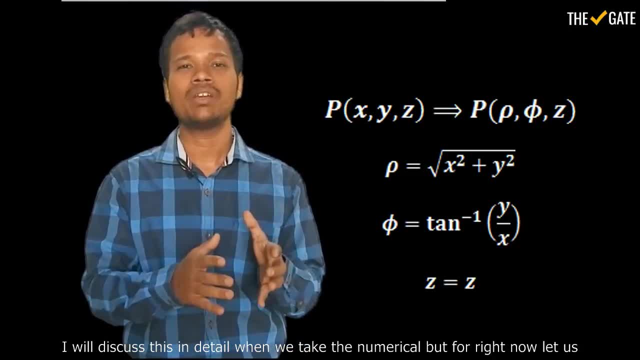 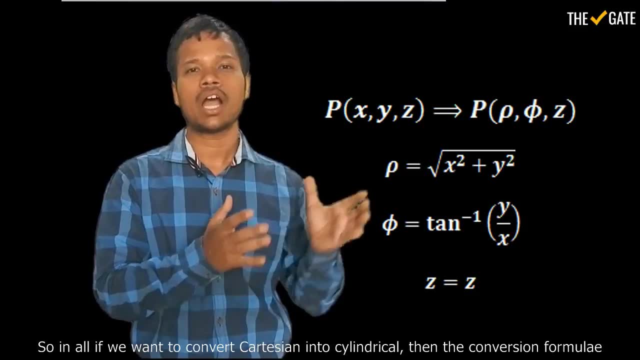 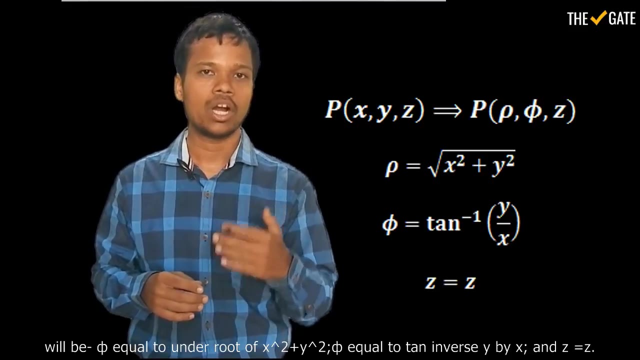 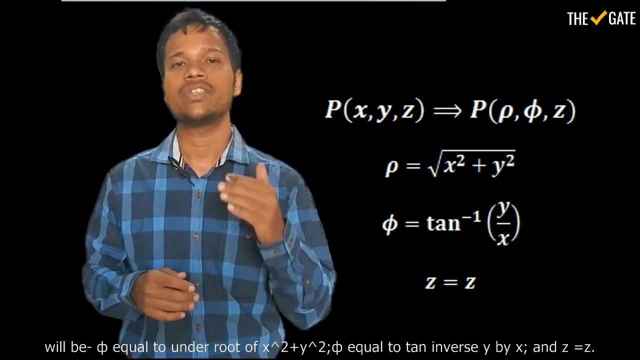 take the numericals, but for right now let us remember: phi equal to tan inverse y by x. so in all, if we want to convert cartesian into cylindrical, then the conversion formula will be: rho equal to tan inverse y by x, under root x square plus y square, phi equal to tan inverse y by x and z equal to z. 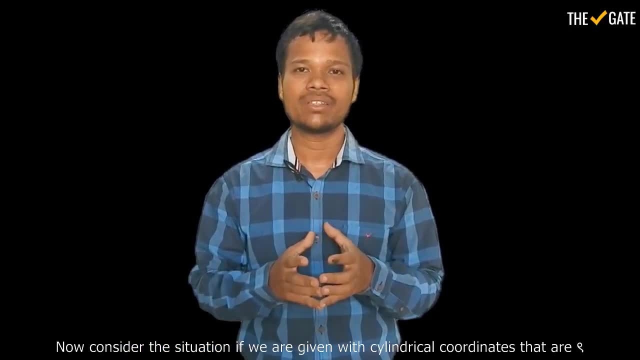 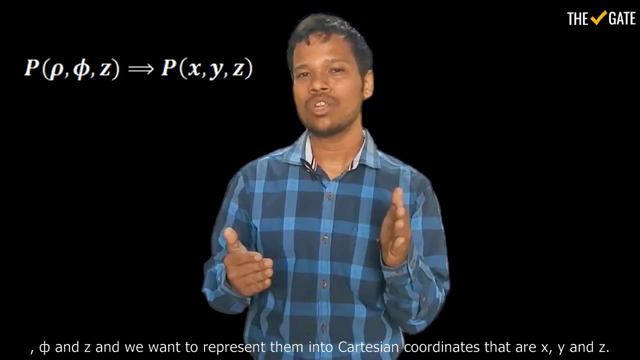 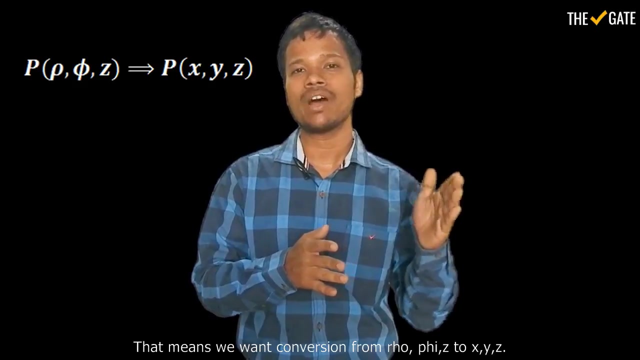 now consider the situation if we are given with cylindrical coordinates that are rho, phi and z and we want to represent them into cartesian coordinates that are x, y and z. that means we want conversion from rho phi, z to x, y, z. once again, consider the situation if we are given with cylindrical coordinates that are rho, phi and z. 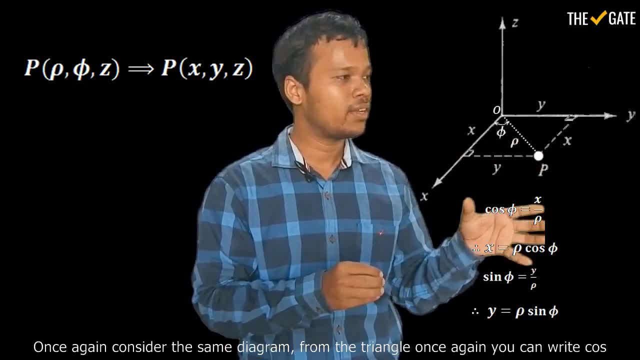 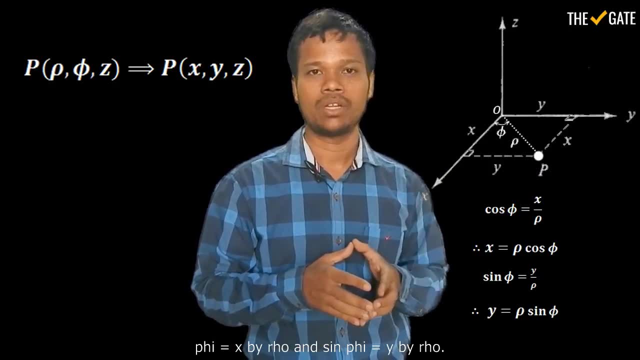 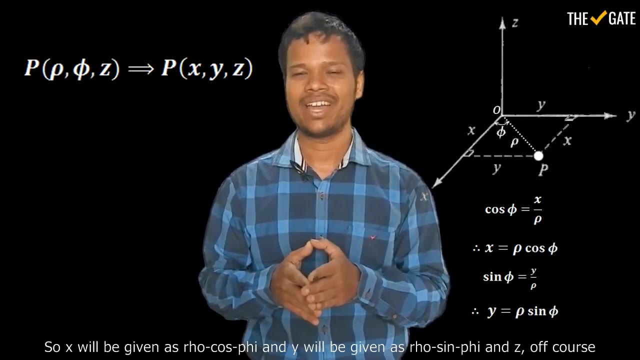 consider the same diagram from the triangle once again. you can write cos phi, equal to x by rho, and sine phi, equal to y by rho. so x will be given as rho, cos phi and y will be given as rho, sine phi and z, of course that will be the same. so the conversion formula for cylindrical. 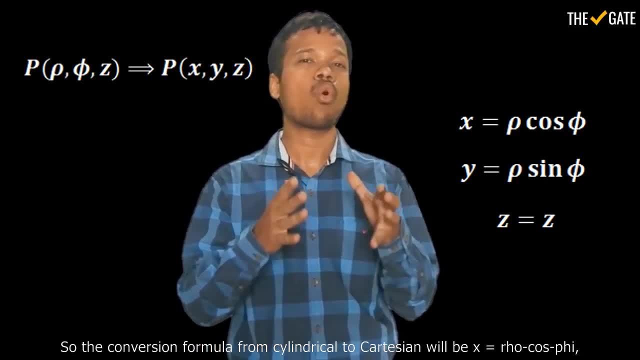 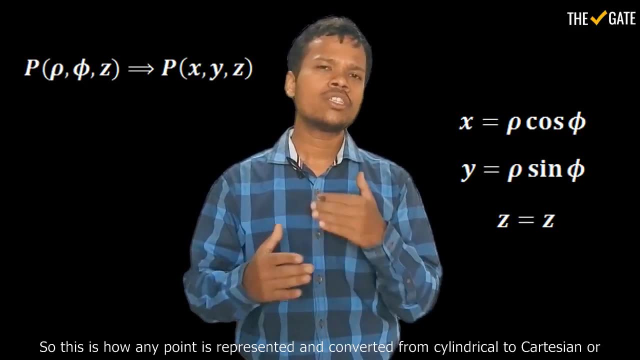 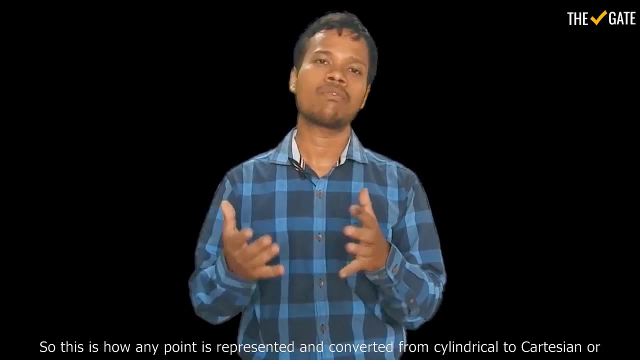 to cartesian will be x equal to rho cos phi, y equal to rho sine phi and z, of course, z will be sine phi and z equal to z. so this is how any point is represented and converted from cylindrical to cartesian or from cartesian to cylindrical. now let us see how any vector from cartesian 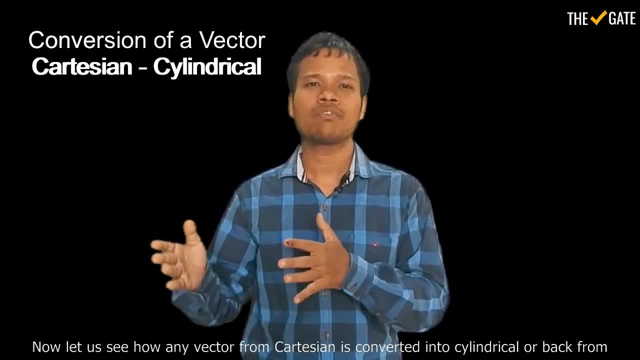 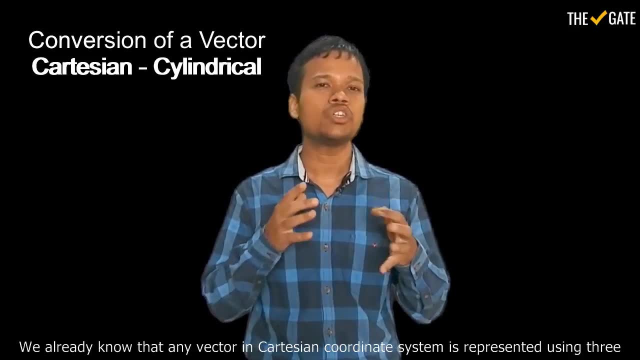 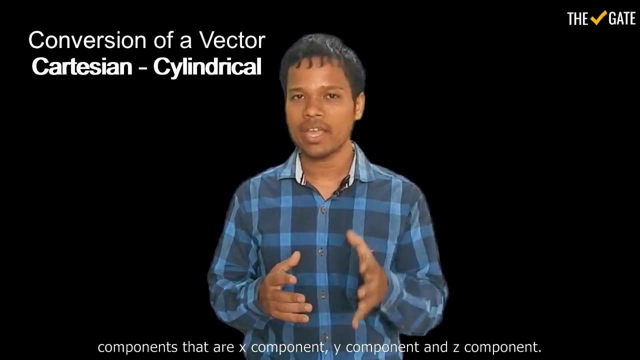 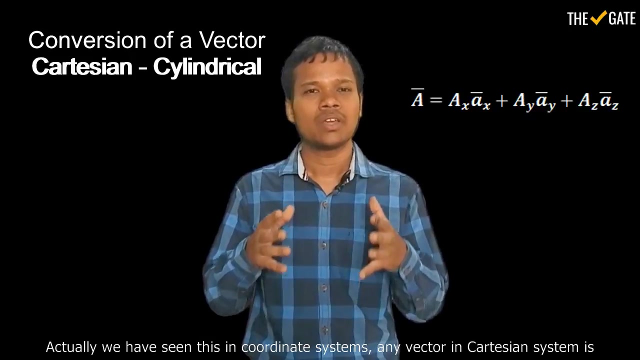 is converted into cylindrical or back from cylindrical to cartesian. we already know that any vector in cartesian coordinate system is represented using three components, that are x component, y component and z component. actually we have seen these in coordinate systems. any vector in cartesian system is represented like this: capital, a x unit vector. 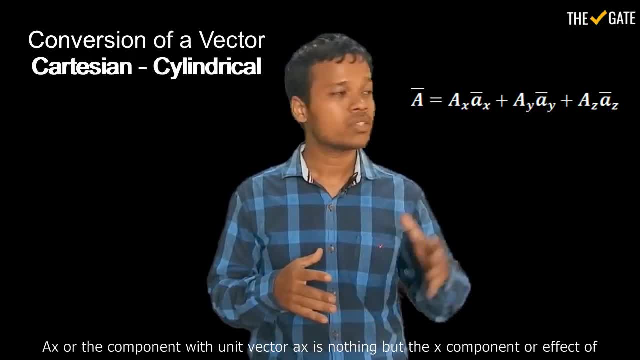 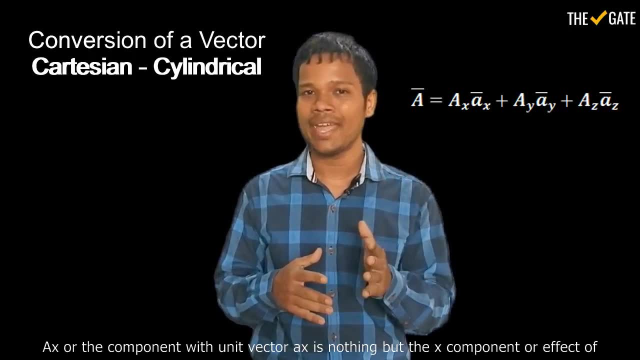 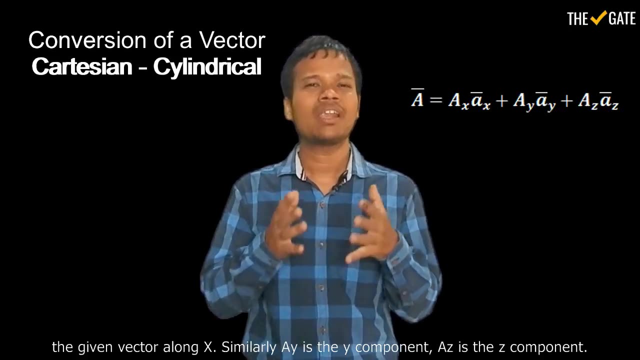 a x plus capital a y. unit vector a y plus capital a z. unit vector a z. capital a- x or component with the unit vector a x is nothing but the x component or effect of the given vector along x. similarly, capital a- y is the y component. capital a- z is nothing but the z component. 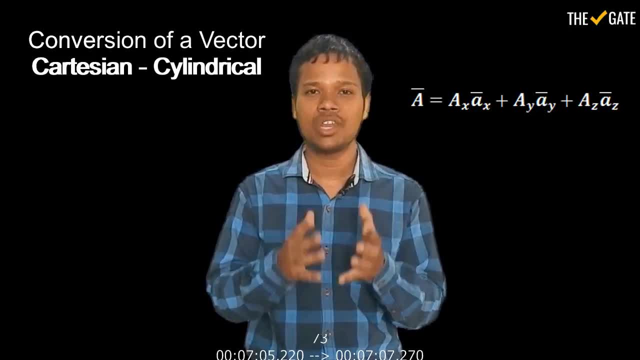 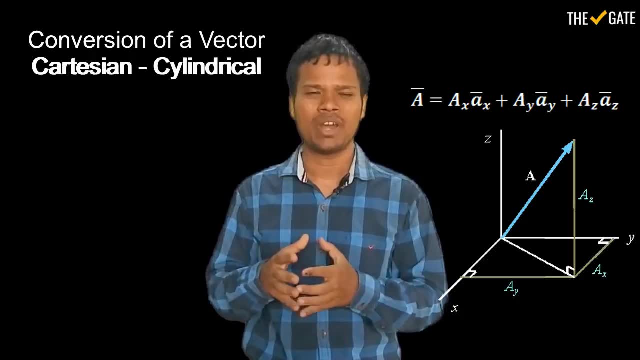 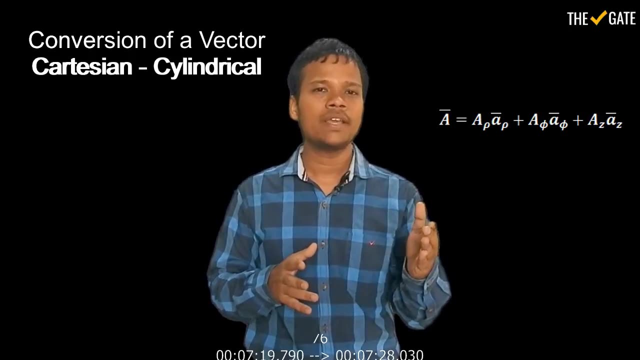 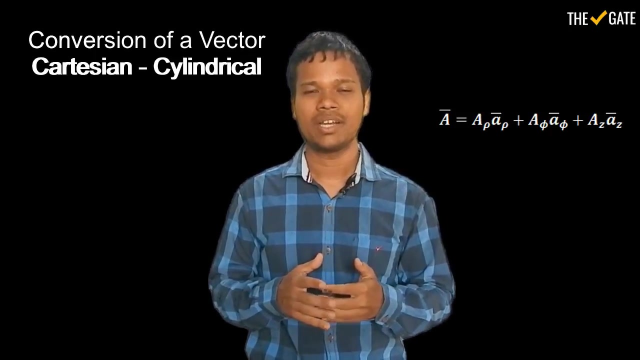 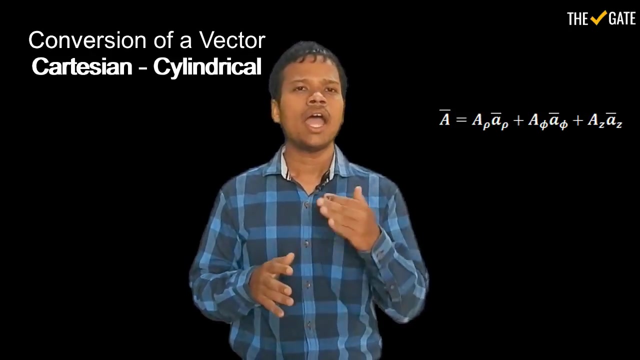 any vector is represented using these three mutually perpendicular components that are: x component, y component and z component. actually, the vector is vector addition of these three components. similarly, in cylindrical coordinates any vector is represented using three mutually perpendicular components that are: row component, phi component and z component. as we have already, 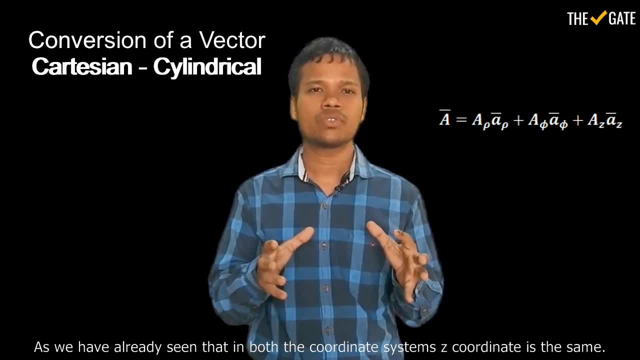 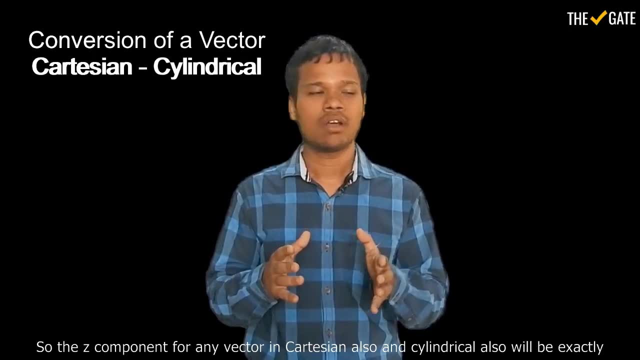 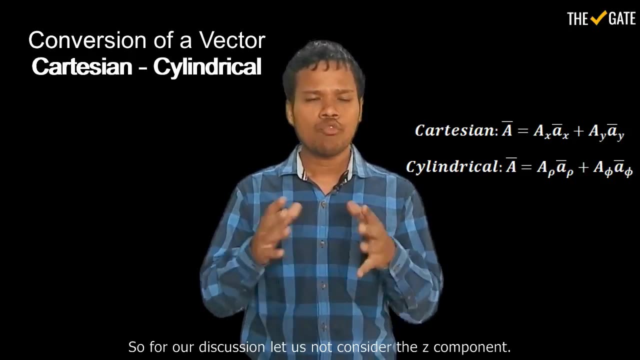 seen that in both the coordinate systems z coordinate is exactly the same. so the z component for any vector, in cartesian also, or in cylindrical also, the z component will be exactly the same. so for our discussion let us not consider the z component as a vector, but let us consider the 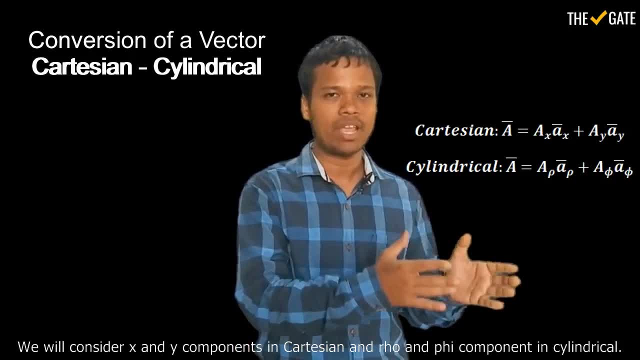 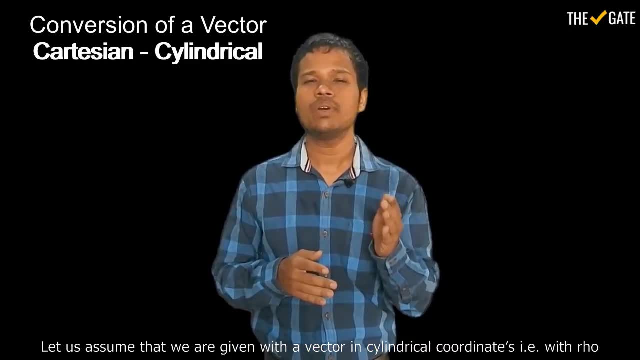 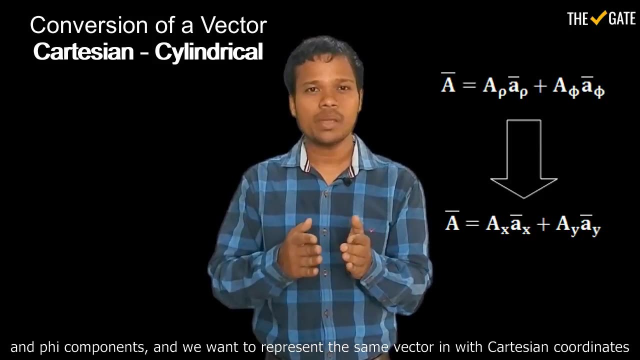 z component. we will consider only x and y component in cartesian and rho and phi component in cylindrical. let us assume that we are given with a vector in cylindrical coordinates, that means with rho and phi components, and we want to represent the same vector in terms of cartesian. 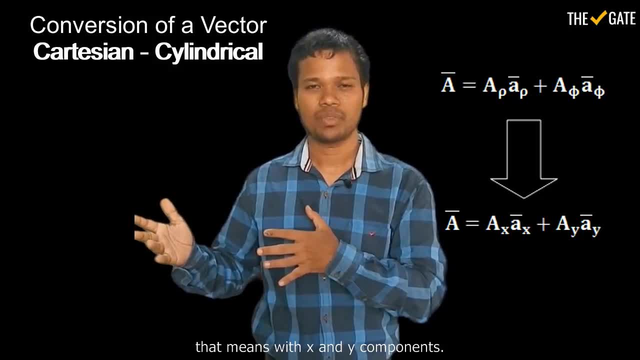 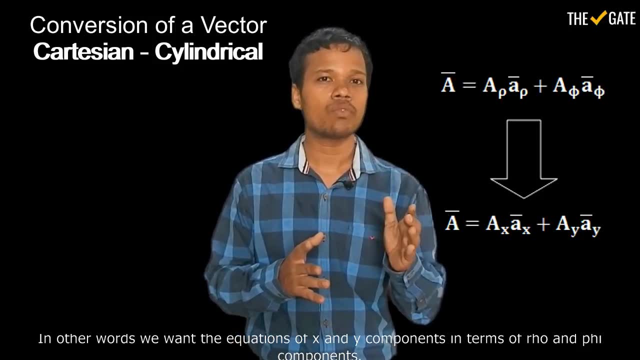 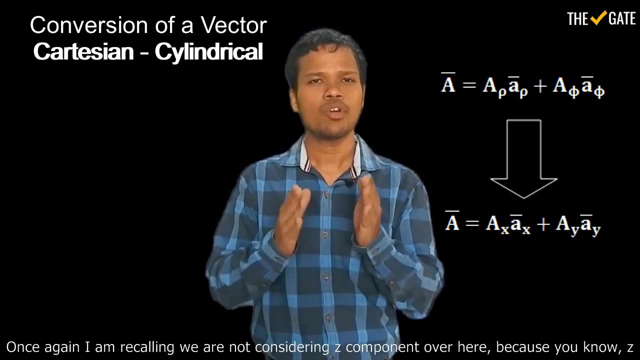 coordinates, that means in x and y components. in other words, we want the equations for x and y in terms of rho and phi components. once again, i am recalling we are not considering z components over here, because you know, z coordinate or z components are going to be the same in both the 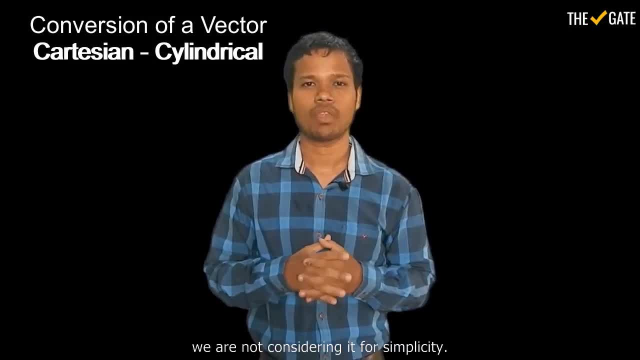 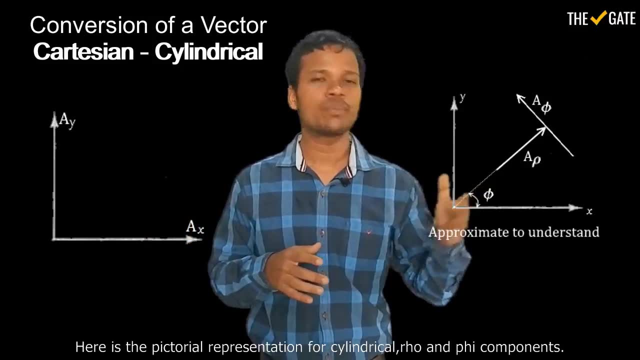 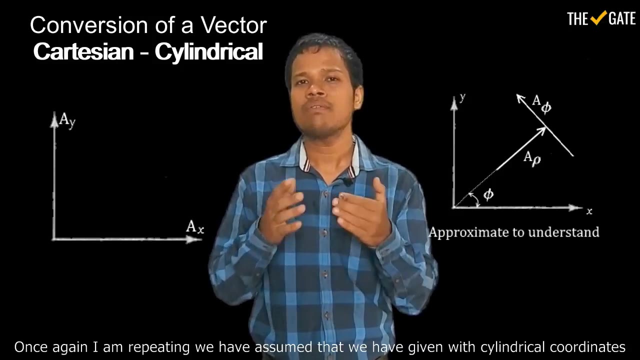 coordinate systems. so we are not considering for simplicity. so here is the pictorial representation for cartesian or x and y components and here is the pictorial representation for cylindrical rho and phi components. once again i am repeating. so we are assuming that we have given width cylindrical coordinates and we want to convert. 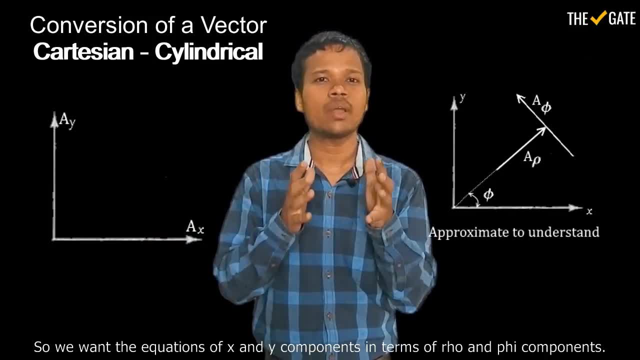 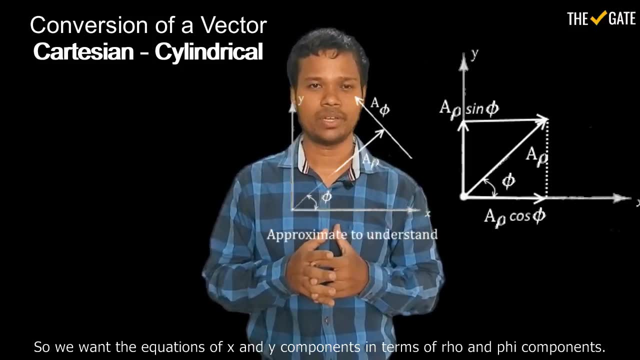 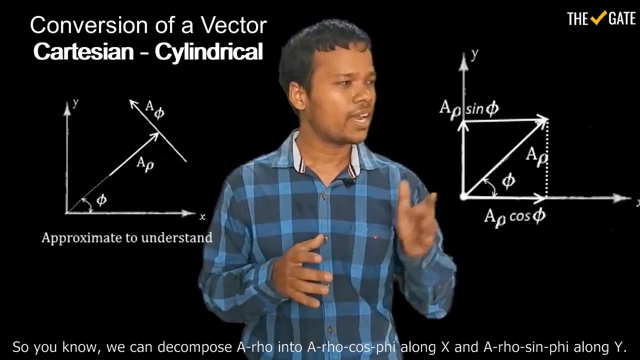 it into cartesian coordinates. so we want the equations for x and y components in terms of rho and phi components. so you know, we can decompose a rho into a rho cos phi along x and a rho sin phi along y. we can also decompose a phi. 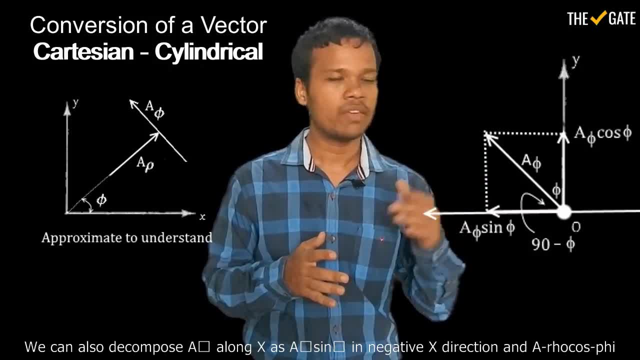 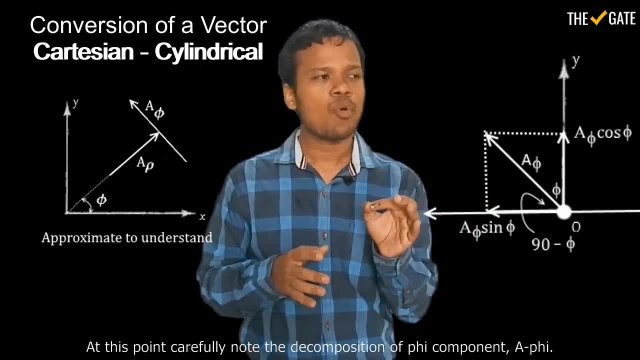 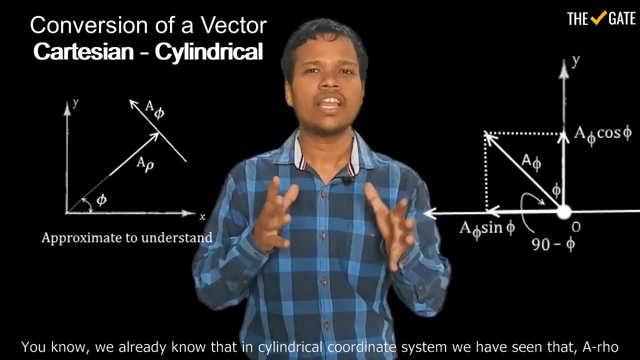 x as a phi sin phi in negative x direction and a phi cos phi along positive y direction. At this point carefully note the decomposition of phi, component a, phi. You know, we already know, that in cylindrical coordinate system we have seen that a rho makes an angle phi. 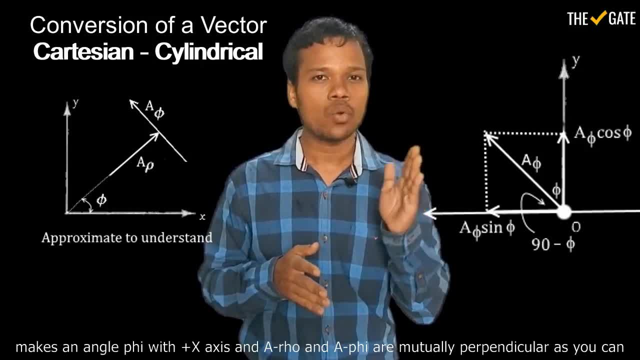 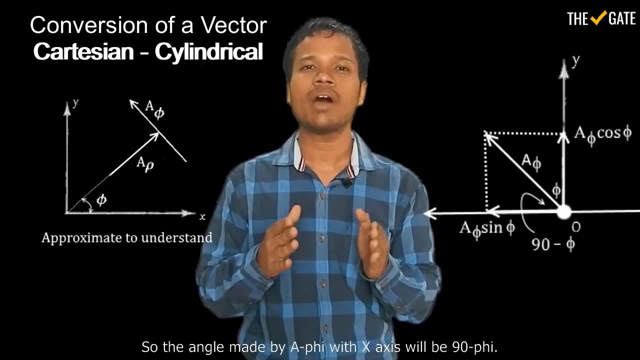 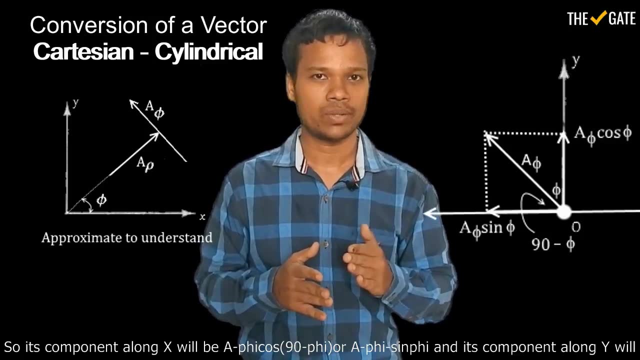 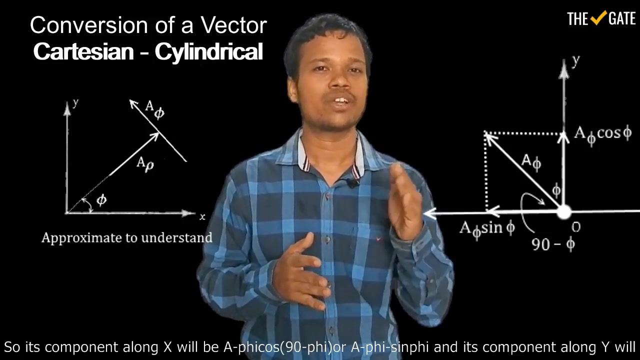 with positive x axis and a rho and a phi are mutually perpendicular, as you can easily say into the diagram. So the angle made by a phi with x axis will be90 minus phi. So its component along x will be a phi cos or a phi sin and its component along y will be 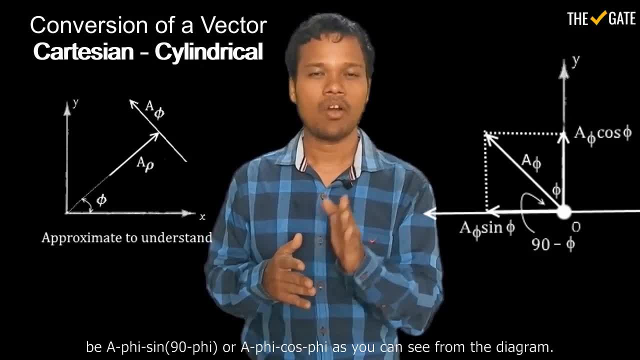 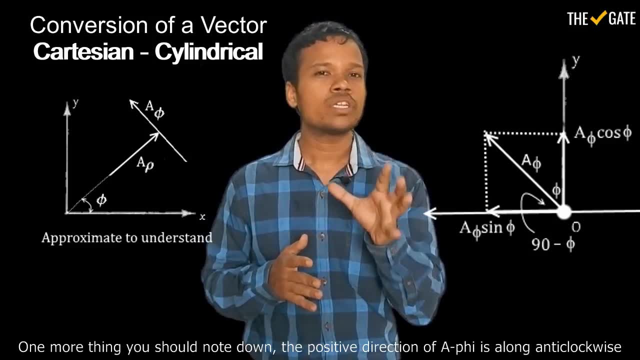 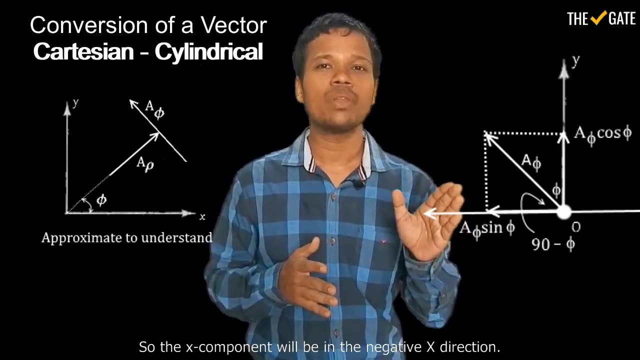 a phi Sin or a regulating space. ok, a phi cos phi, as you can see into the diagram. One more thing you should note down: the positive direction of a phi is along anticlockwise direction, as shown in the diagram. So the x component will be in negative x direction. So you can easily see from the diagram we have decomposed. 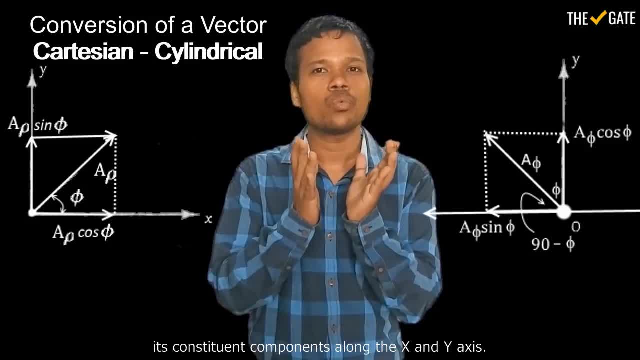 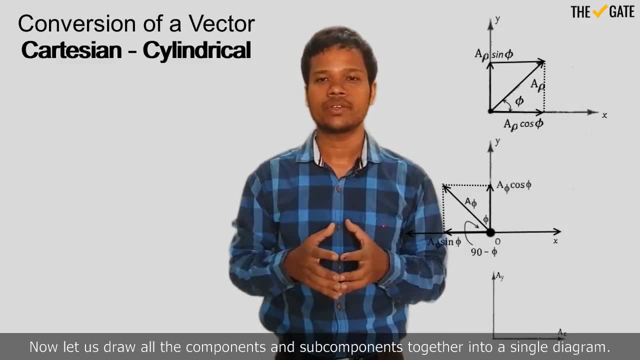 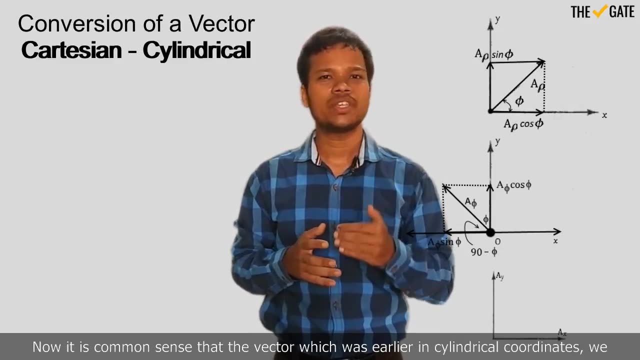 rho and phi components into its constituent components along the x and y axis. Now let us draw all the components and subcomponents that we have discussed together into a single diagram. Now it is common sense that the vector, which was earlier in cylindrical coordinates, we want to 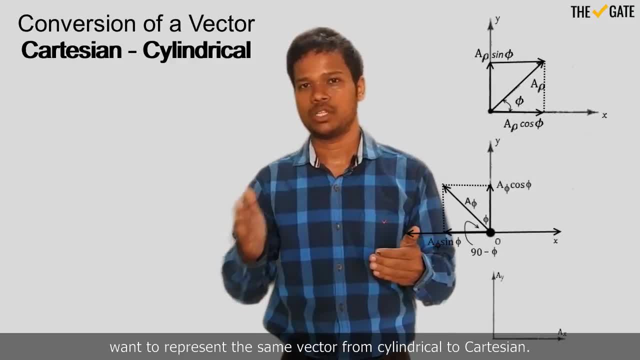 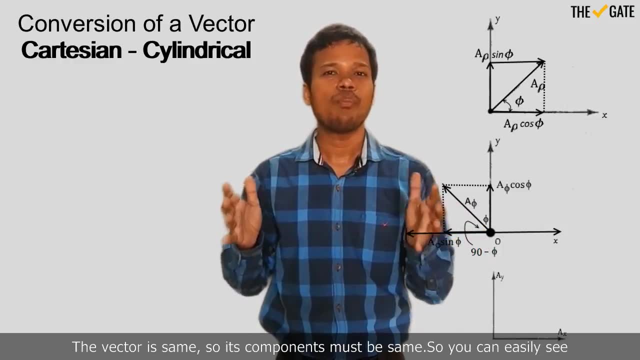 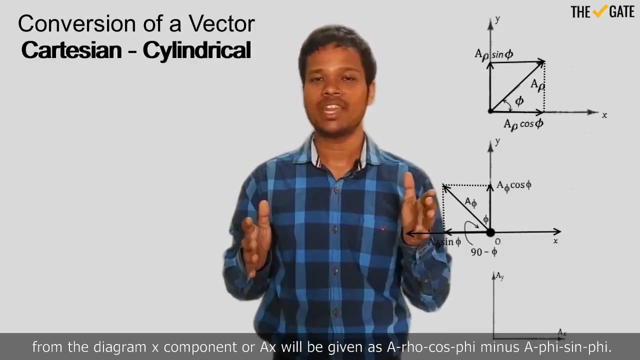 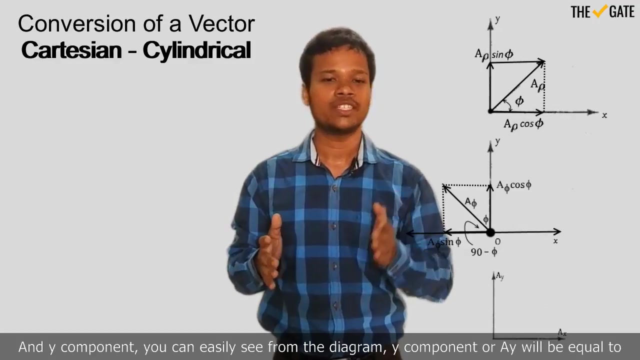 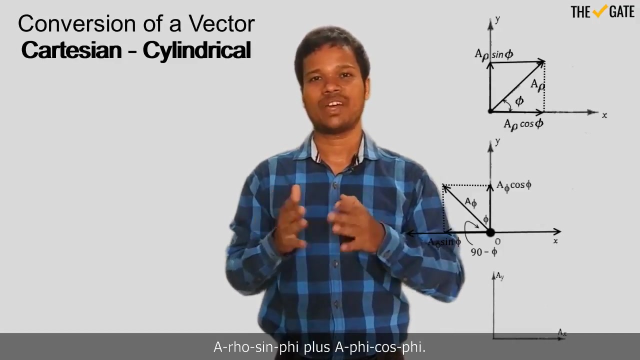 represent the same vector from cylindrical to cartesian. We want just representation from cylindrical to cartesian. the vector is same, So its components must be same. So you can easily see from the diagram x component, or ax. x will be given as a rho cos phi minus a phi sin phi and y component. you can easily see from the diagram y component, or a: y will be equal to a rho sin phi plus a phi cos phi. 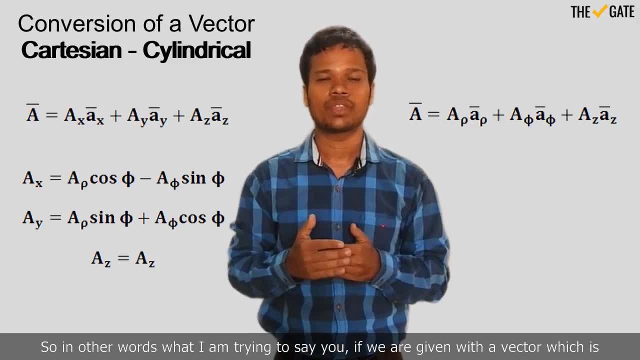 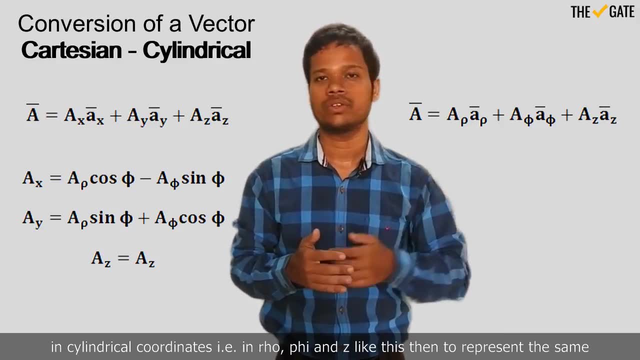 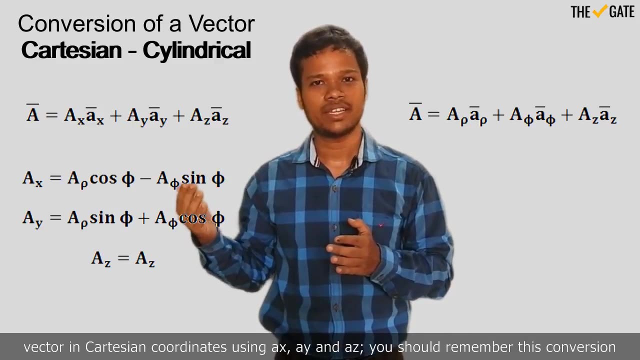 So, in other words, what I am trying to say: you, if we are given with a vector which is in cylindrical coordinates- that means in rho, phi and z, like this, then to represent this same vector into cartesian coordinates using a, x, a y and a z. you should remember this conversion. 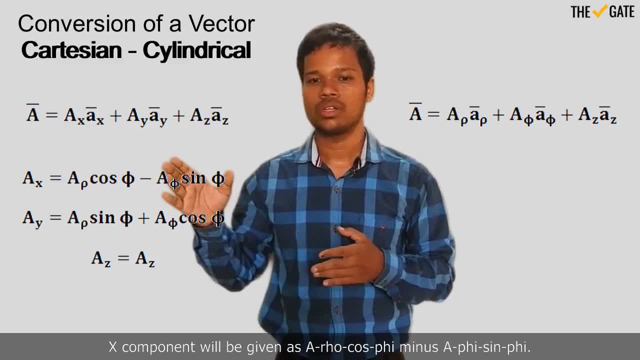 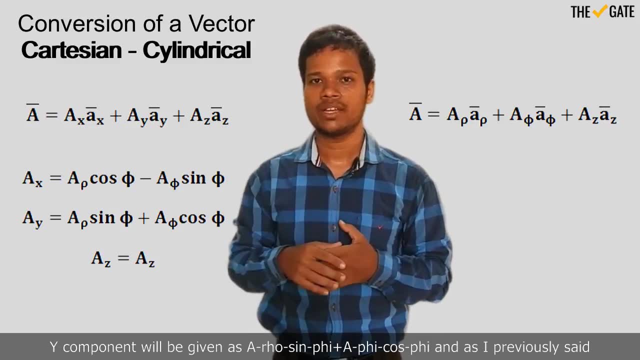 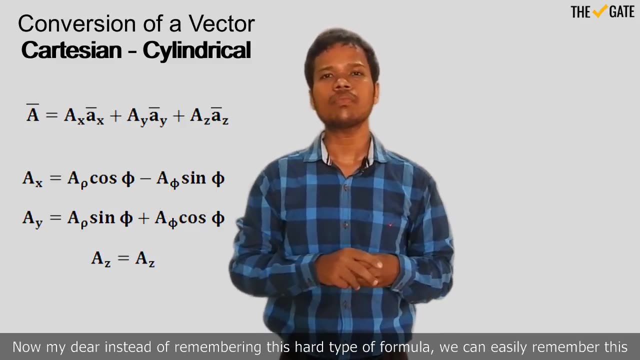 formula: x component will be given as a rho cos phi minus a phi sin phi, y component will be given as a rho sin phi plus a phi cos phi and, as we previously said, z component will be the same in cylindrical also and cartesian also. Now, my dear, instead of remembering this hard type of formula, 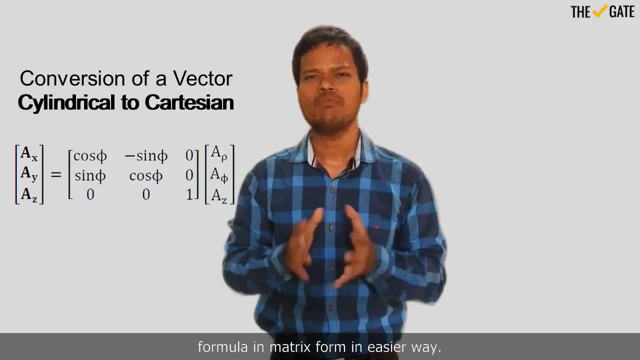 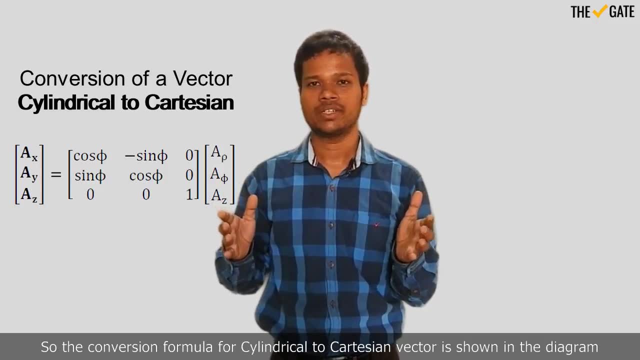 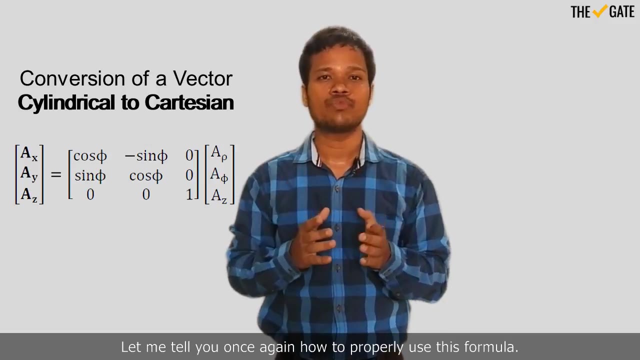 I can easily remember this formula in matrix form in a very easier way. So the conversion formula for cylindrical to cartesian vector is shown in the diagram like this. Let me tell you once again how to properly use this formula. Note that this formula is used when we want to. 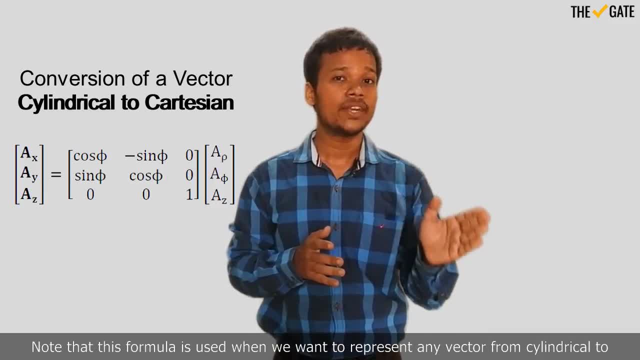 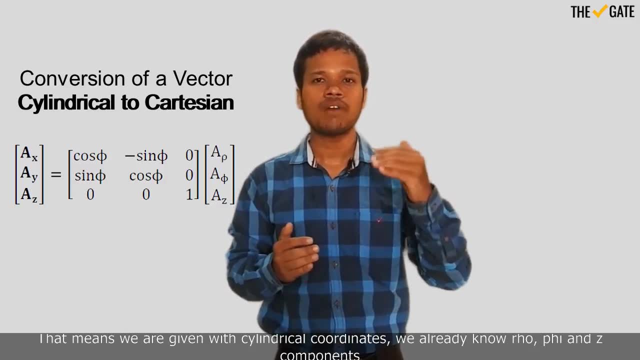 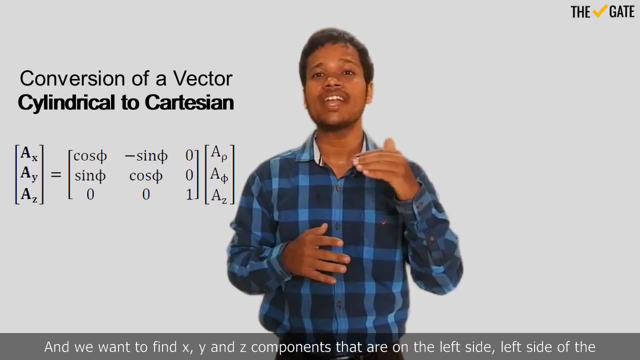 represent any vector from cylindrical to cartesian. That means we are given with a cylindrical coordinates, coordinates we already know: rho, phi and z. that should be put on the right hand side of the matrix formula and we want to find x, y and z components that are on the left side of the 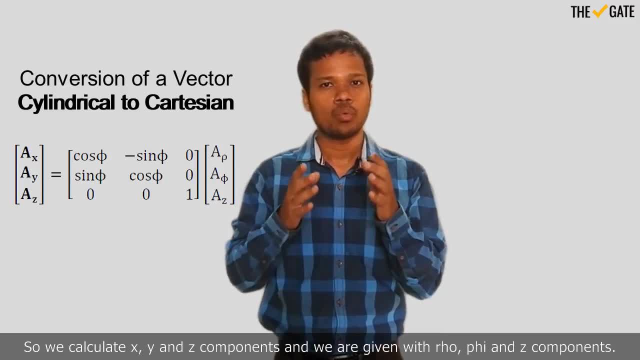 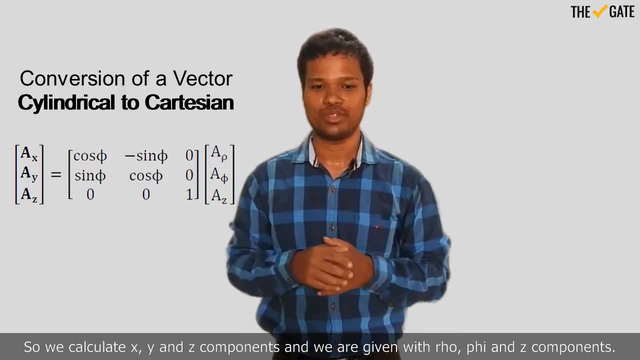 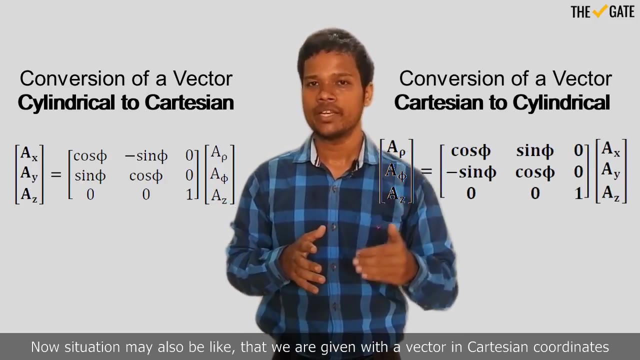 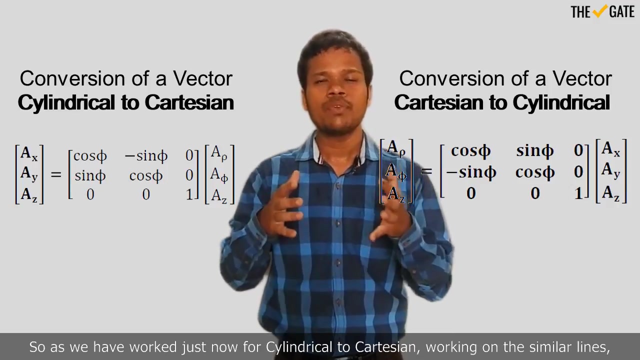 left side of the equation. So we calculate x, y and z component and we are given with rho, phi and z components. Now situation may also be like that we are given with a vector in cartesian coordinates and we want to represent that vector into cylindrical coordinates. So as we have worked, 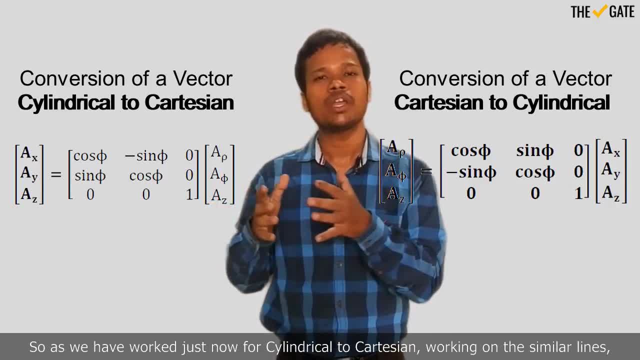 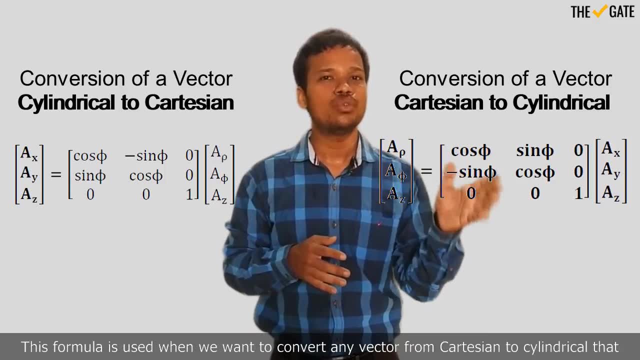 just now for cylindrical to cartesian. working on the similar lines, we may get the formula as shown in here. This formula is used when we want to convert any vector from the vector to the vector. So we want to convert any vector from the vector to the vector. 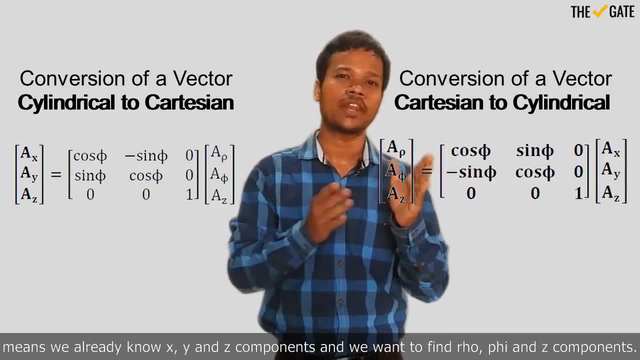 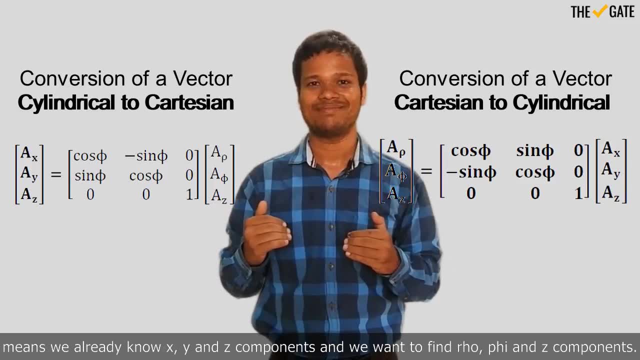 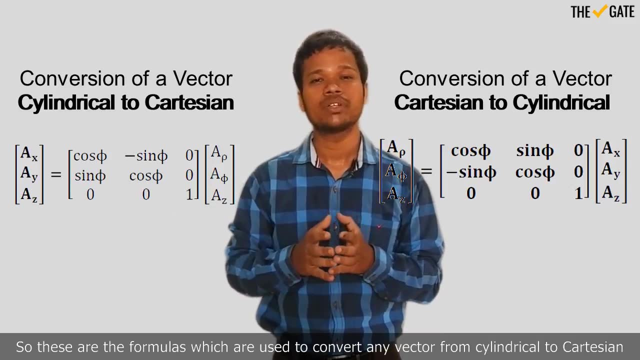 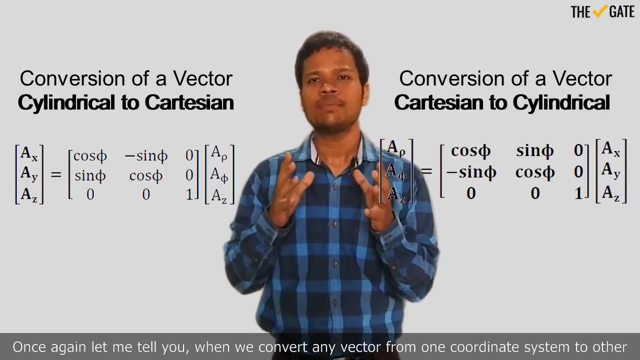 from cartesian to cylindrical. That means we already know x, y and z components and we want to find rho, phi and z component. So these are the formula which are used to convert any vector from cylindrical to cartesian or from cartesian to cylindrical. Once again, let me tell you: 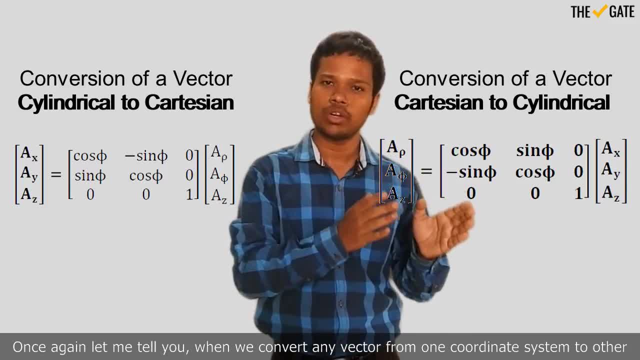 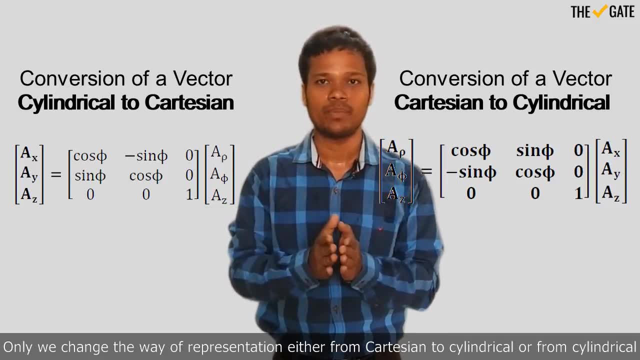 when we convert any vector from one coordinate system to other coordinate system, we are given with a vector from the vector to the vector. So we want to convert any vector from one coordinate system to another coordinate system, The vector isn't going to be changed. Vector remains same. Only we change the way of representation, either from. 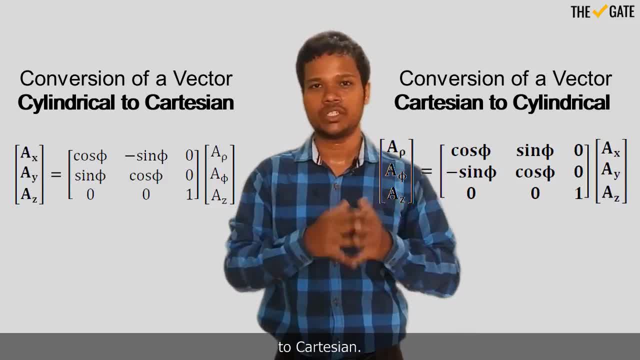 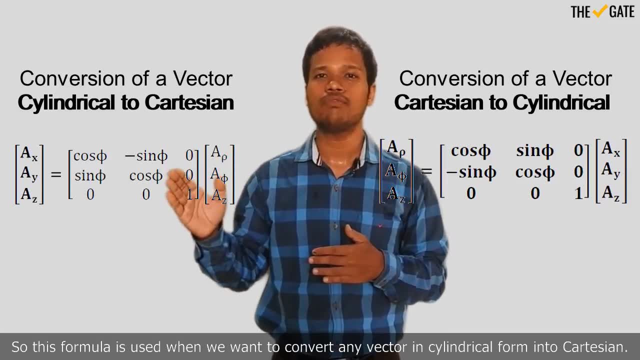 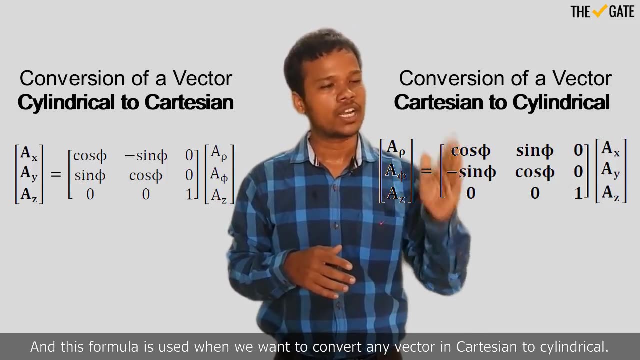 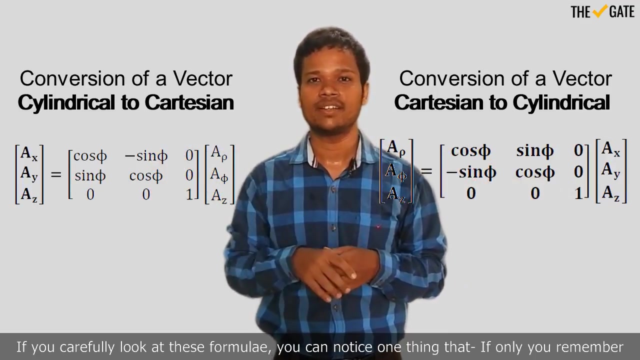 cartesian to cylindrical or from cylindrical to cartesian. So this formula is used when we want to convert any vector in cylindrical form into cartesian and this formula is used when we want to convert any vector in Cartesian to cylindrical. if you carefully look at this formula, you can notice one thing: that if only you remember one formula. 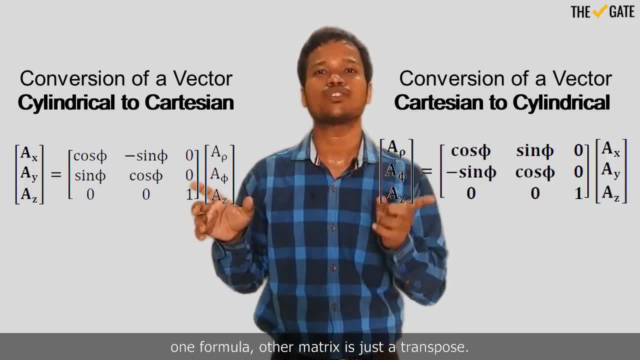 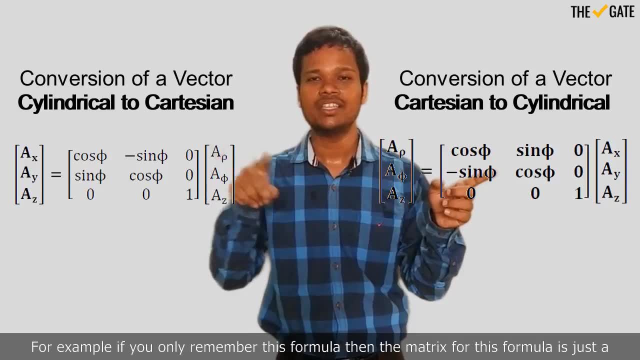 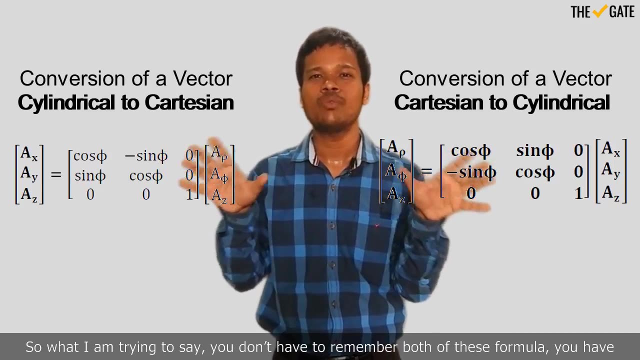 other matrix is just the transpose. for example, if you only remember this formula, then the matrix for this formula is just a transpose. so what I'm trying to say: you don't have to remember both of these formula. you have to remember only one formula, either from cylindrical to Cartesian or from Cartesian to 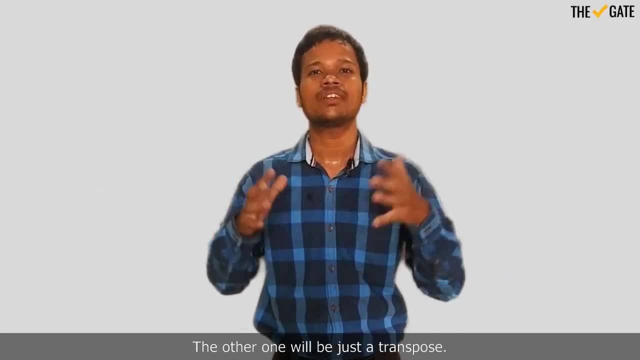 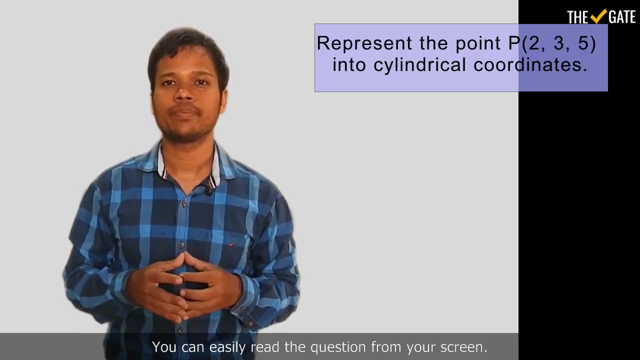 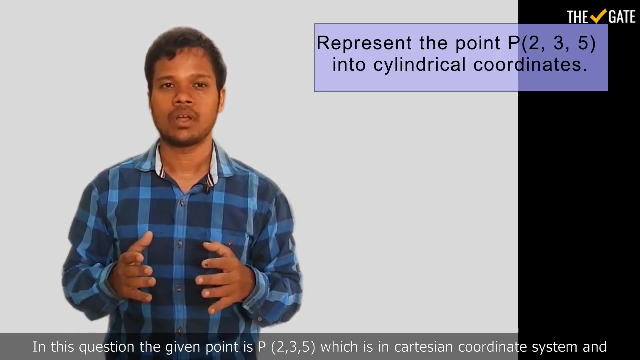 cylindrical, the other one will be just the transpose. okay, let us now solve few numericals. you can easily read the question from your screen. in this question, the given point is P, 2, 3, 5, which is in Cartesian coordinate system, and we are supposed to be able to solve this question in the following way. 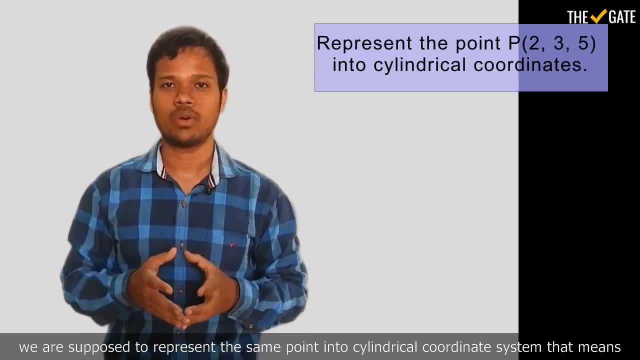 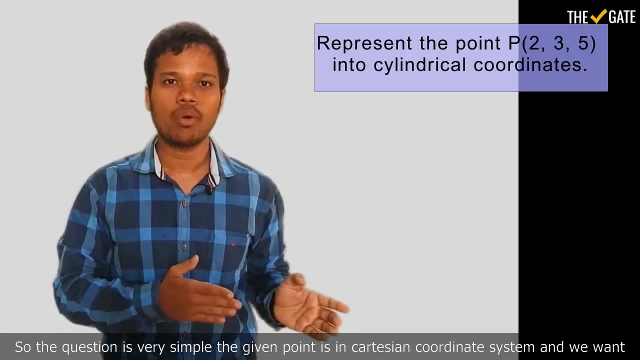 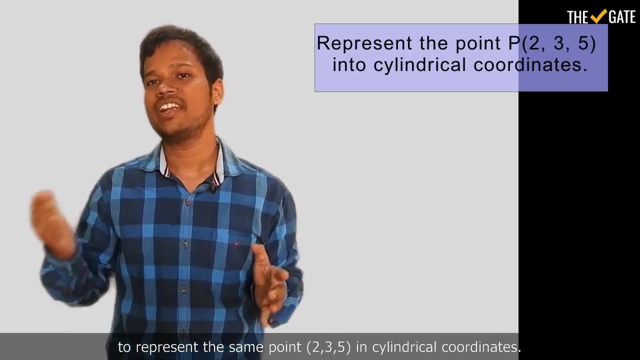 suppose to represent the same point into cylindrical coordinate system. that means in Rho, Phi and Z. so the question is very simple. the given point is in Cartesian coordinate system and we want to represent the same point- 2, 3, Phi, U- in cylindrical coordinates. now, as we know that in cylindrical coordinates any 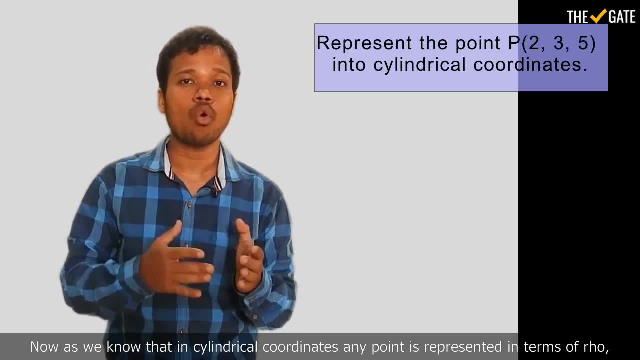 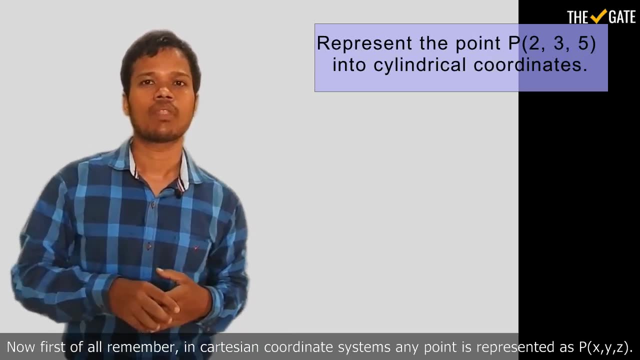 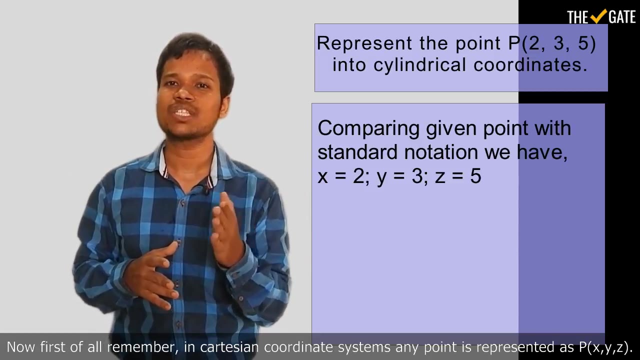 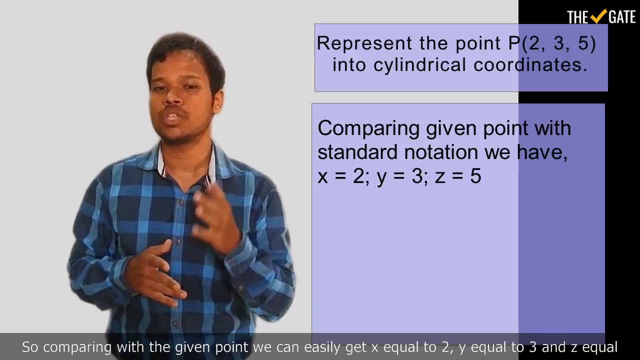 point is represented in terms of Rho, Phi and Z. so in this question we have to find Rho, Phi and Z. now, first of all, remember, in Cartesian coordinate systems any point is represented as P, X, Y, Z. so, comparing with the given point, we can easily get X equal to 2, Y equal to 3 and Z equal to 5. now we already also. 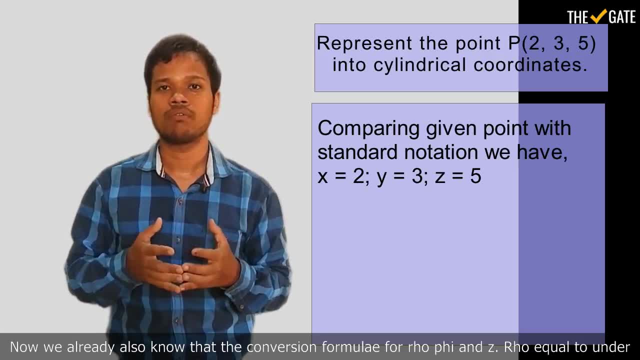 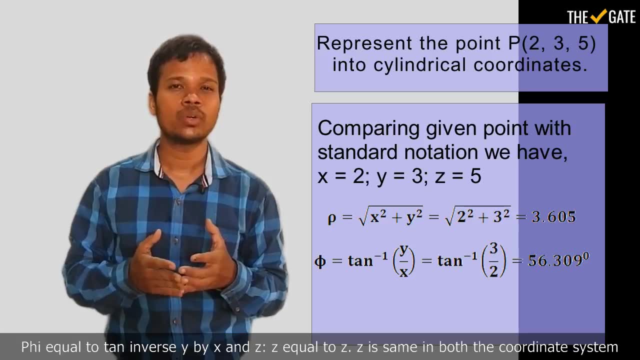 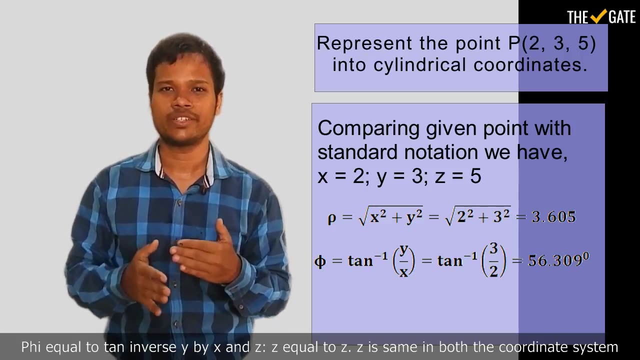 know that the conversion formulae for Rho, Phi and Z, Rho, equal to under root of X square plus Y square. Phi equal to tan inverse Y by X and Z, Z equal to Z. Z is same in both the coordinate system. so whatever Z given is Cartesian, that the same Z will also be. 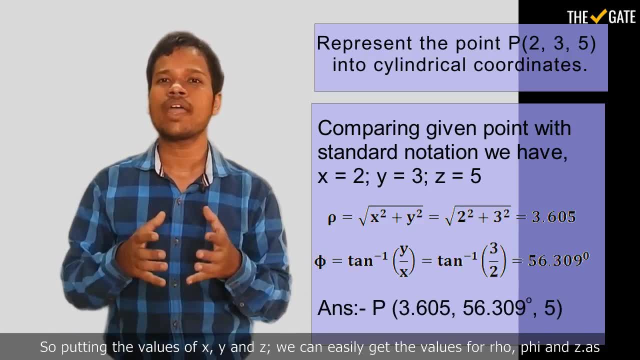 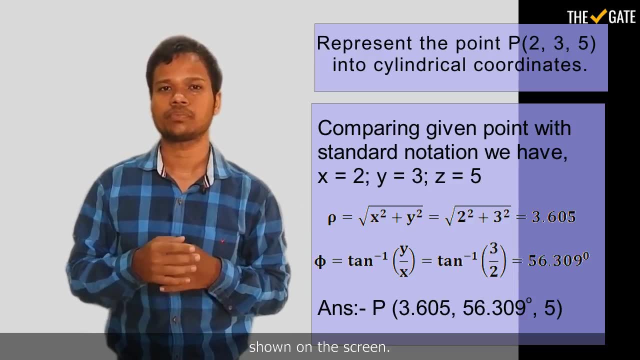 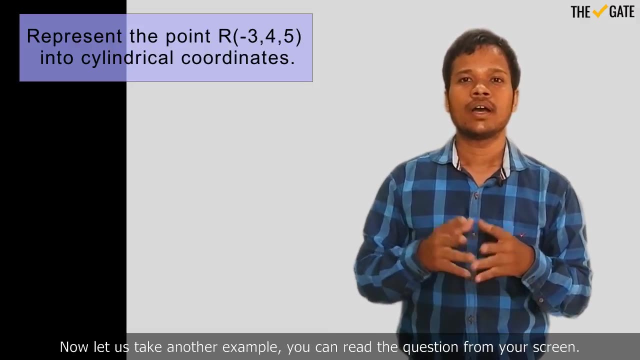 there in cylindrical, so putting the values of X, Y and Z. we can easily get the values for Rho, Phi and Z as shown on the screen. now let us take another example. you can read the question in the following way: the question from your screen. in this question, the given point is R minus 3, 4. 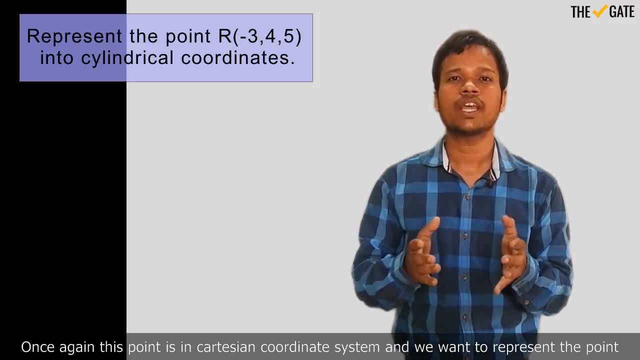 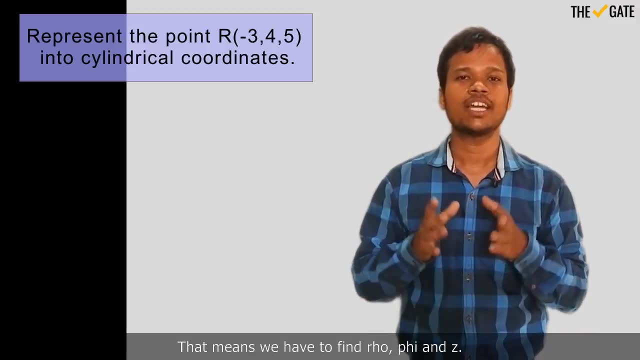 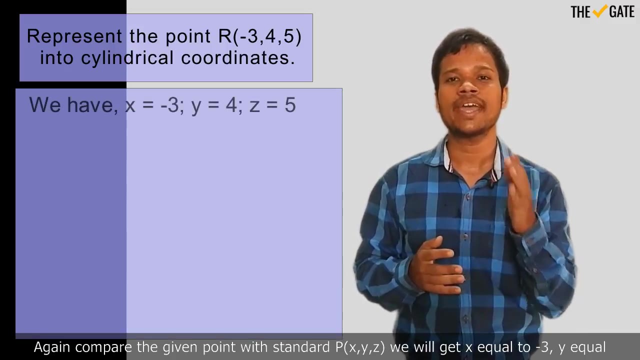 5. once again, this point is in Cartesian coordinate system and we want to represent this point into cylindrical coordinates. that means we have to find out Rho, Phi and Z again. compare the given point with standard point P, X, Y, Z. we will get X equal to minus 3. 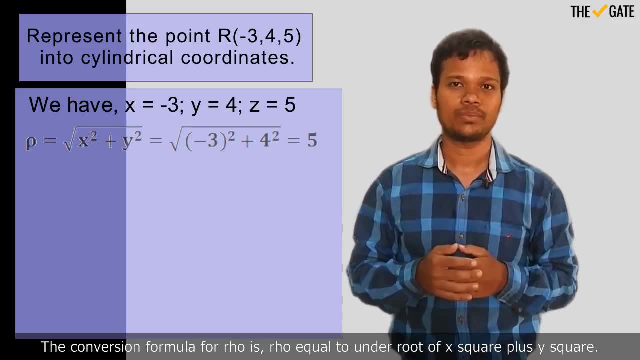 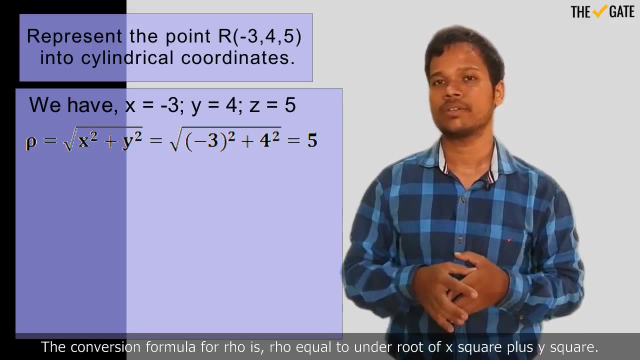 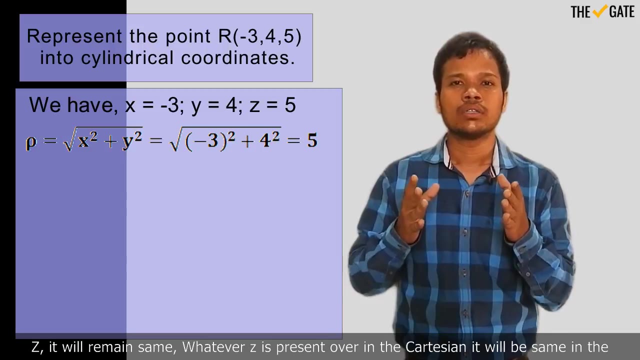 equal to 4 and Z equal to 5. the conversion formula for Rho is Rho equal to under root of X square plus Y square. so putting the values for X and Y, we get easily. Rho as shown in the screen. Z- it will remain same to whatever be Z present over in the Cartesian. it will be same in the. 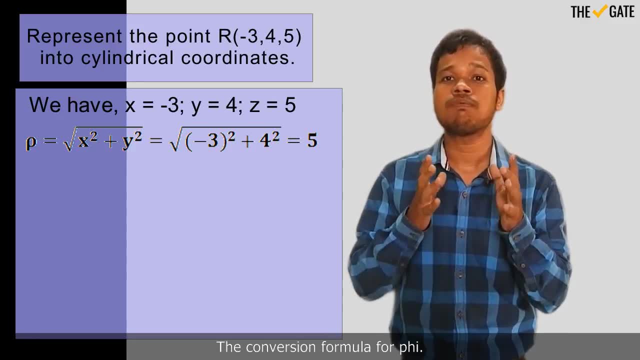 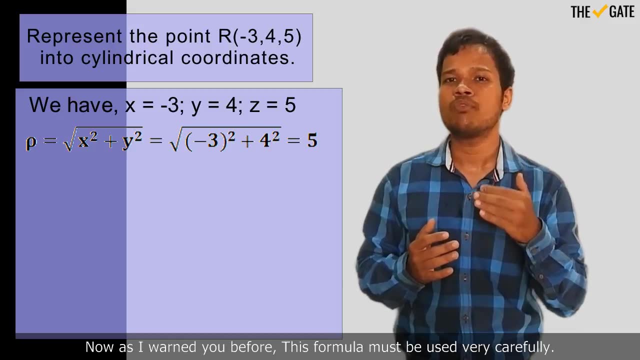 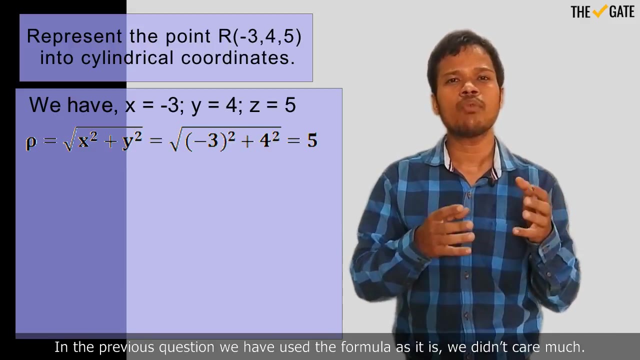 cylindrical. also the conversion formula for Phi: Phi equal to tan, inverse Y and Z equal to 4 and Z equal to 5, Y by X. now, as I warned you before, this formula must be used very carefully. in the previous question we have used the formula as it is. we didn't care much. 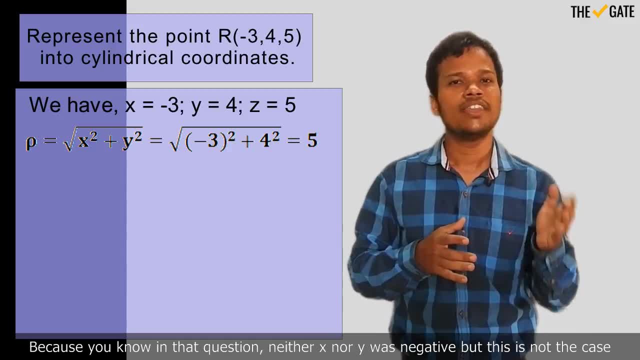 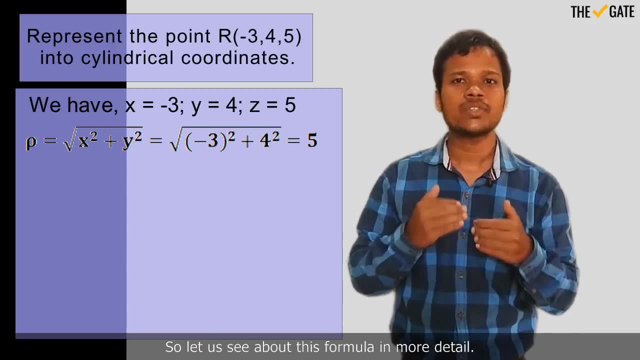 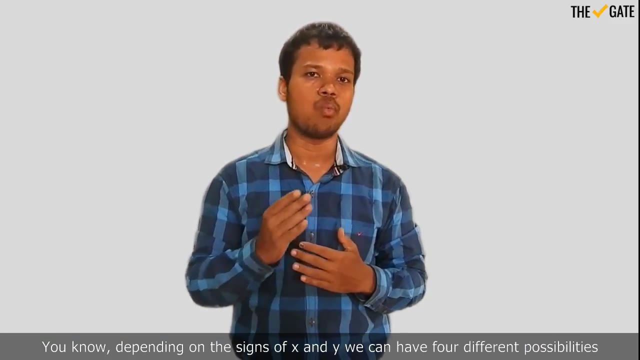 because you know, in that question neither X nor Y was negative, but this is not the case with this question. so let us see about this formula in more detail. you know, depending on the signs of X and Y, we can have four different possibilities for a point. point can be within first quadrant or 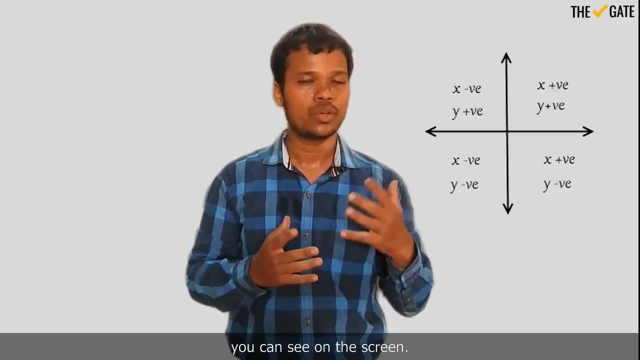 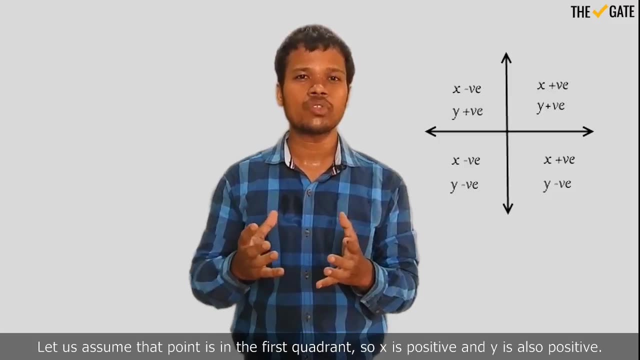 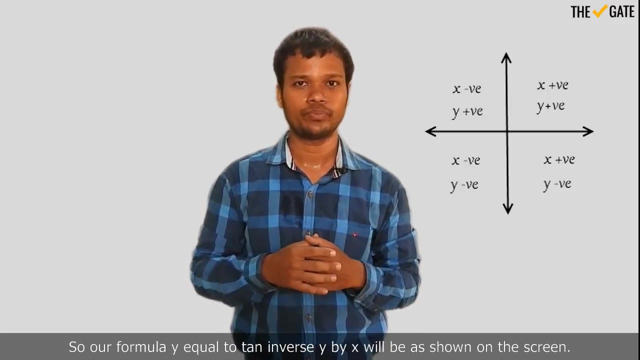 second or third or fourth quadrant of X? Y plane, as you can see on the screen. let us assume that point is in the first quadrant of X? Y plane. so X is positive and Y is also positive. so our formula Phi, equal to tan, inverse Y by X, will be as shown on the screen. now let us 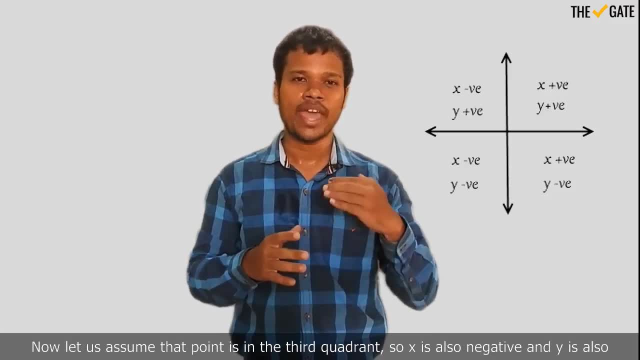 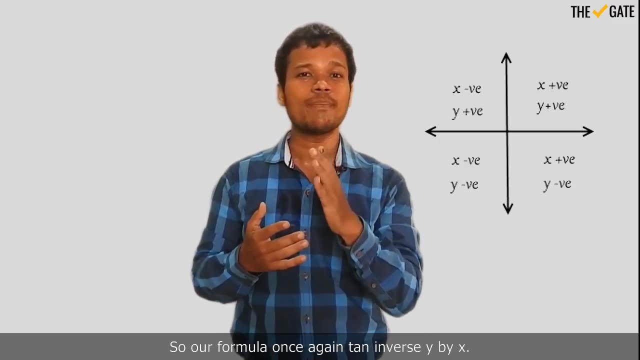 assume that point is in the third quadrant. so X is also negative and Y is also negative. so our formula once again: Phi equal to tan inverse Y by X minus minus get cancelled. so Phi would be like this as you can see on the screen, but if you look, 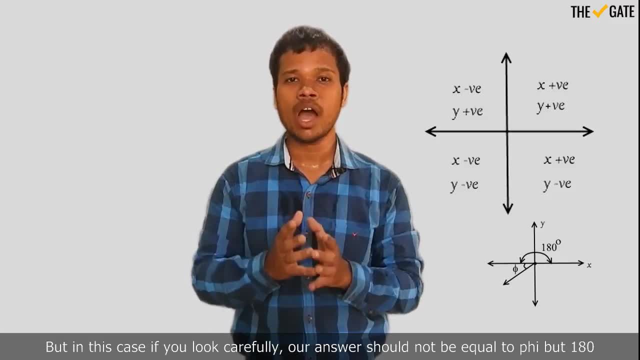 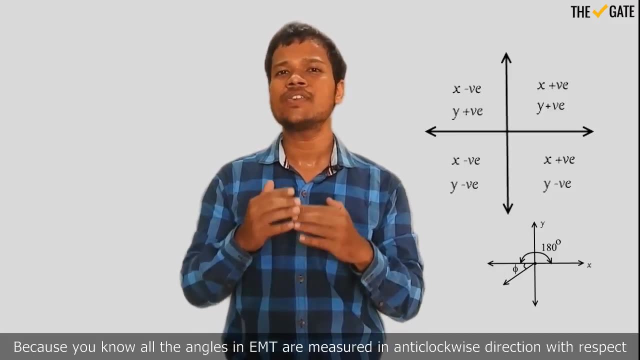 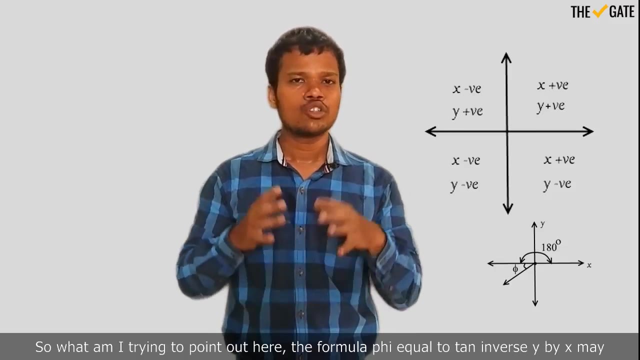 carefully. in this case, our answer for Phi should not be equal to Phi, but 180 plus Phi, because you know, all the angles in EMT are measured in anti-clockwise direction with respect to positive x-axis. so So what I am trying to point out here, the formula phi equal to tan inverse y by x may. 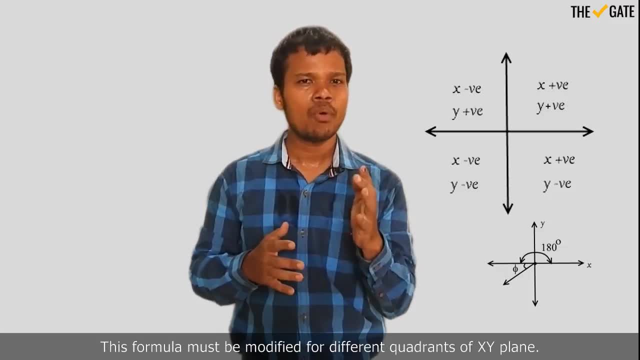 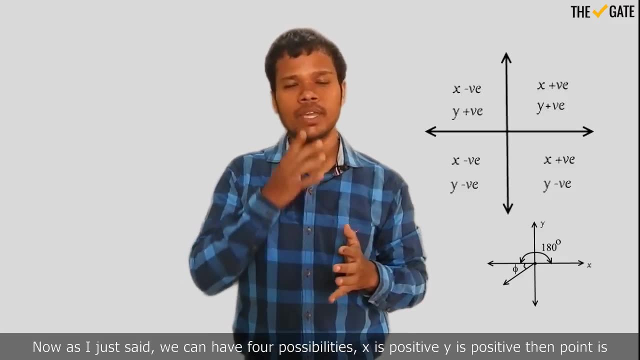 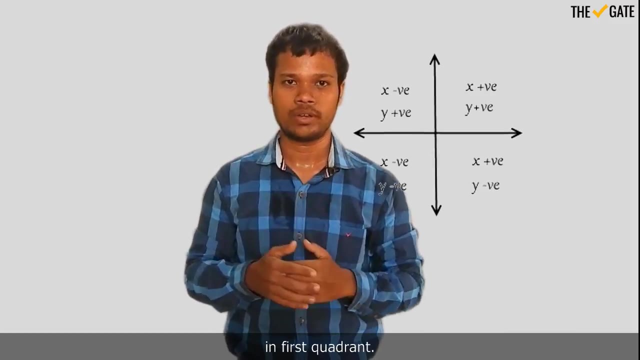 or may not give you the correct answer. This formula must be modified for different quadrants of xy plane. Now, as I just said, we can have four possibilities. x is positive, y is positive, then point is in first quadrant. x is negative, y is positive, point is in second quadrant. 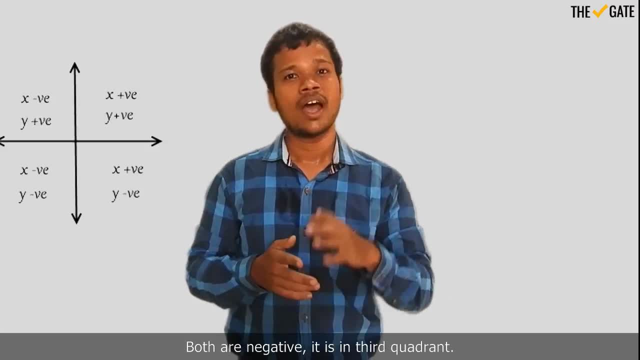 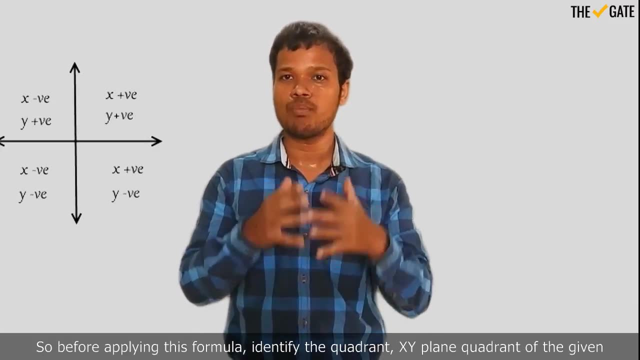 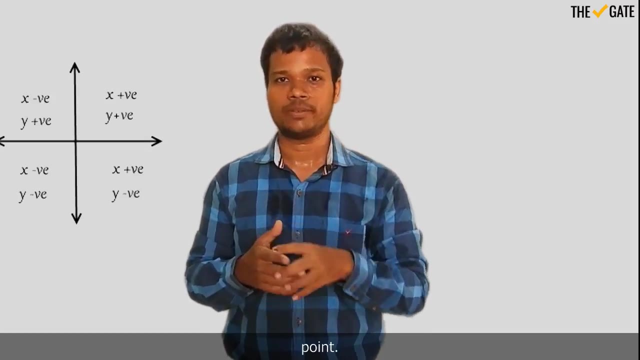 Both are negative. it is in third quadrant, X is positive but y is negative, then it is in fourth quadrant. So, before applying this formula, identify the quadrant xy plane quadrant of the given point. Then, after identifying the quadrant for the point, apply the formula phi equal to tan. 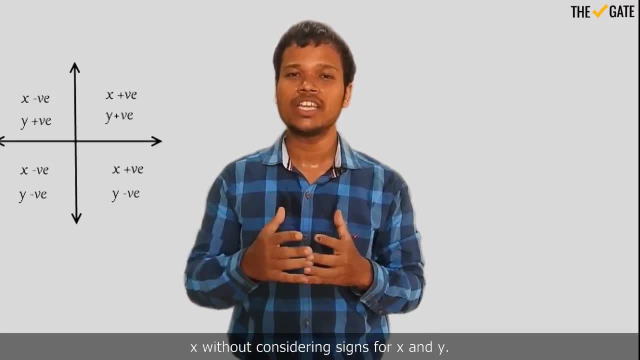 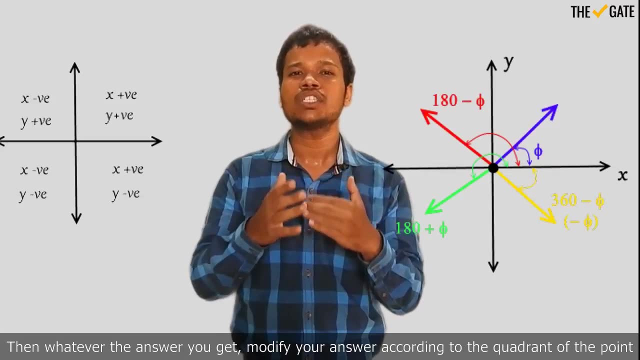 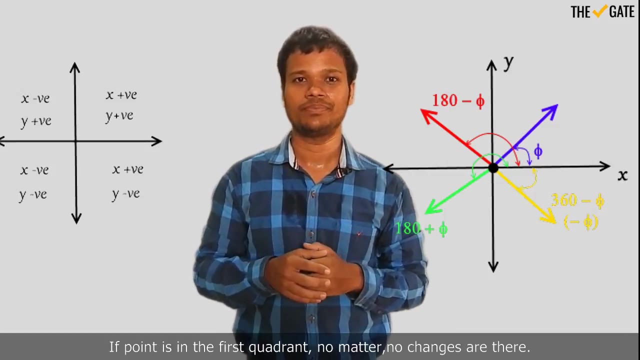 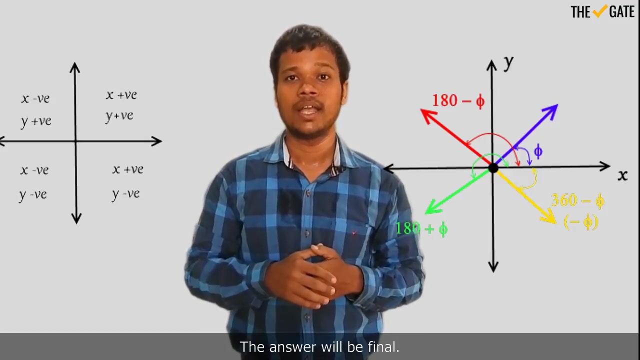 inverse y by x, without considering the signs for x and y, Just considering. Consider magnitudes and apply the formula. Then, whatever the answer you get, modify your answer according to the quadrant of the point as shown on your screen. If point is in the first quadrant, no matter. no changes are there. the answer will be final. 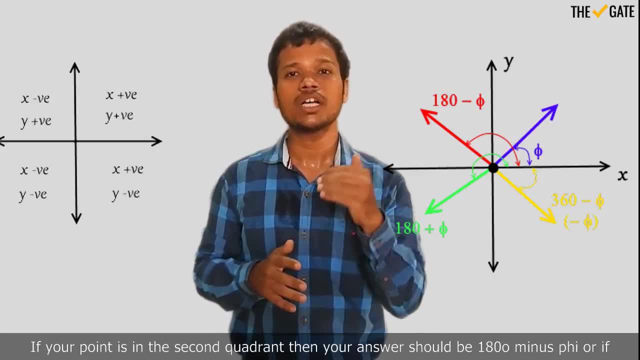 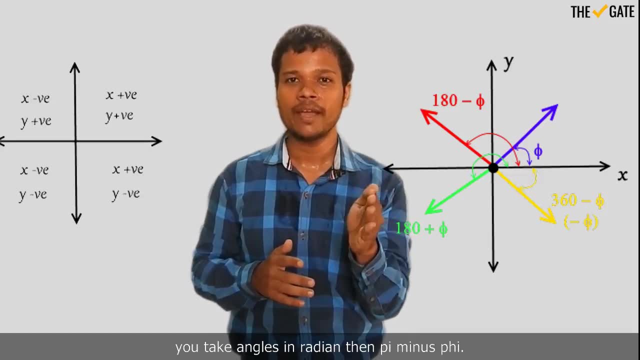 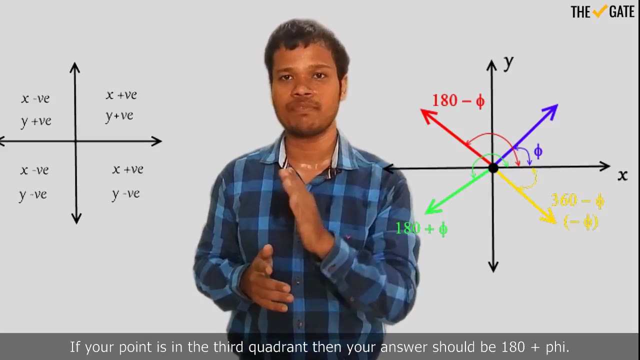 If your point is in the second quadrant, then your answer should be 180 degree minus phi, or if you take angle in radians, then pi minus phi. If your given point is in the third quadrant, then your answer should be 180 plus phi. 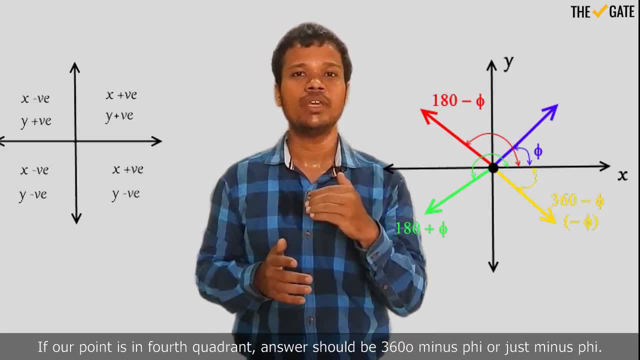 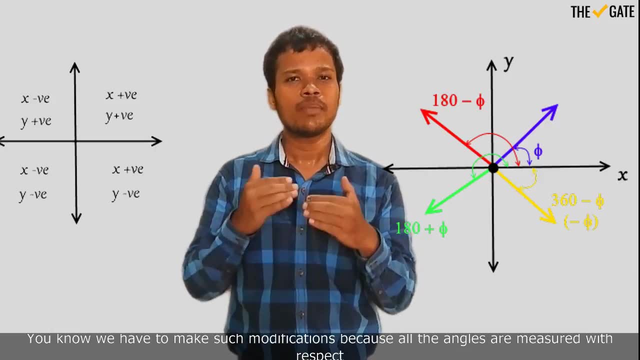 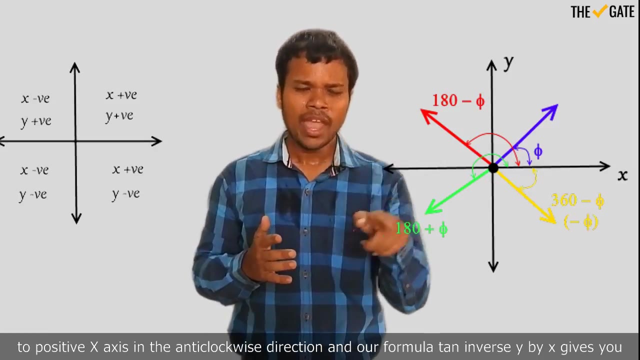 If our point is in fourth quadrant, then our answer should be 360 degree minus phi or just minus phi. You know we have to make such modifications because all the angles they are measured with respect to positive x-axis in the anticlockwise direction and our formula phi equal to tan. 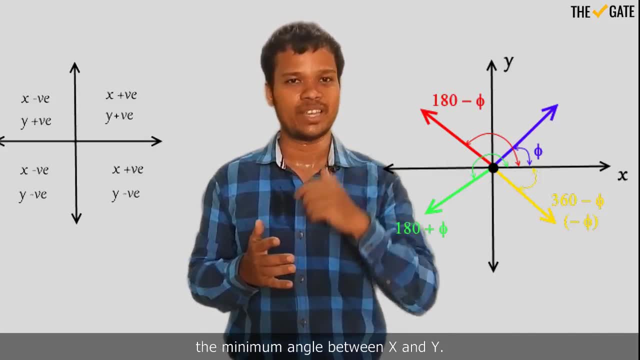 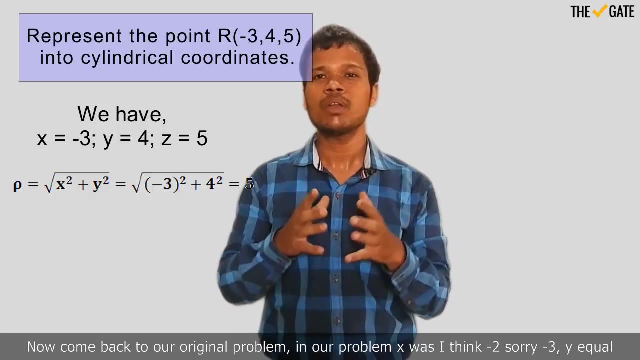 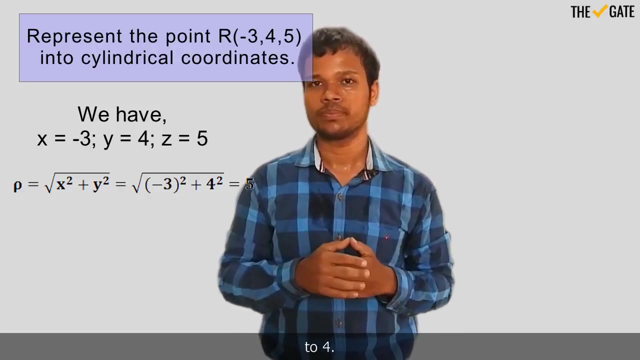 inverse y by x Gives you the minimum angle between x and y. That's why such modifications are required. Now come back to our original problem. In our problem, x was, I think, minus 2, sorry, minus 3,- y equal to 4.. 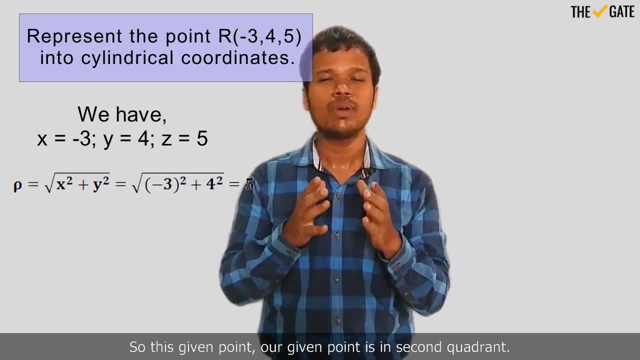 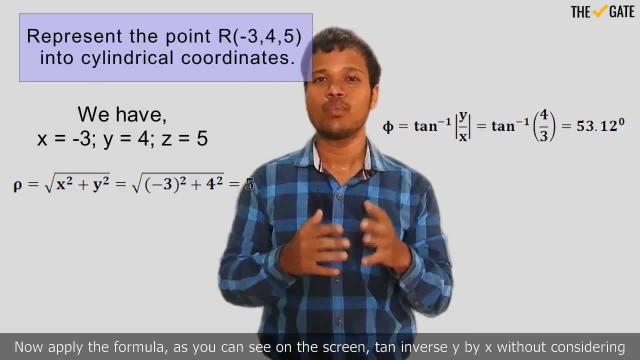 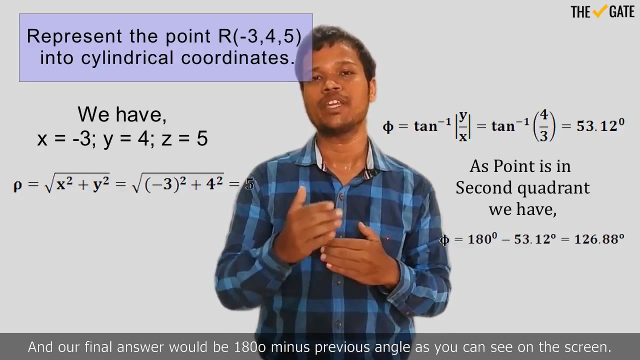 So this given point, our given point, is in second quadrant. Now apply the formula, as you can see on the screen: tan inverse y by x, without considering the sign, And our final answer would be 180 degree minus previous angle, as you can see on the 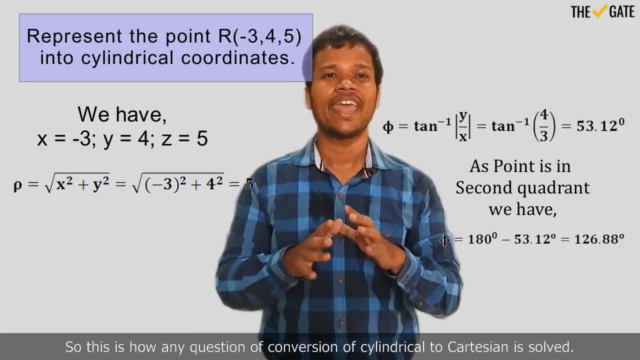 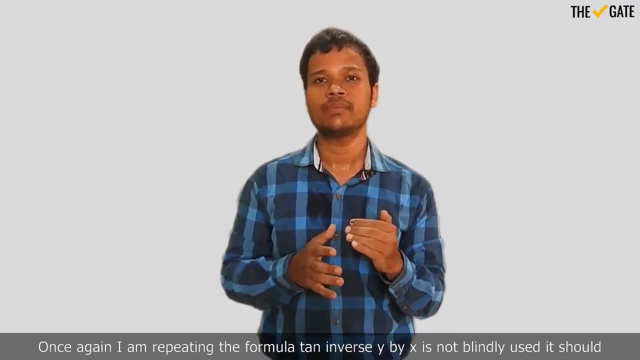 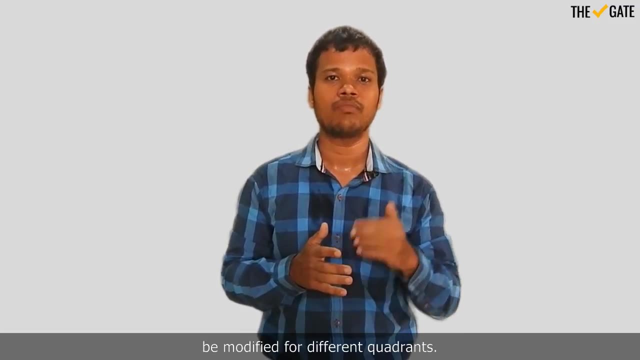 screen. So this is how any question of conversion of cylindrical to Cartesian is solved. Once again I am repeating. the formula phi equal to tan inverse y by x is not blindly used. it should be modified for different quadrants. Consider the next question. as you can see on the screen, 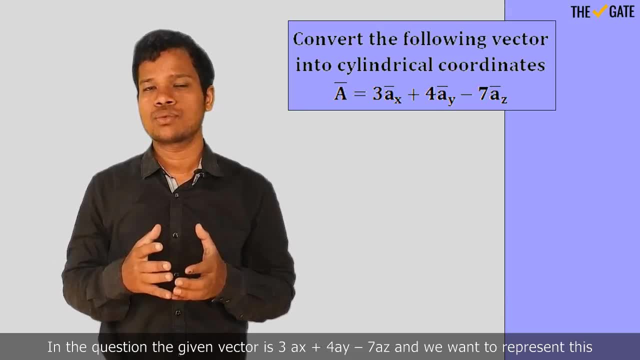 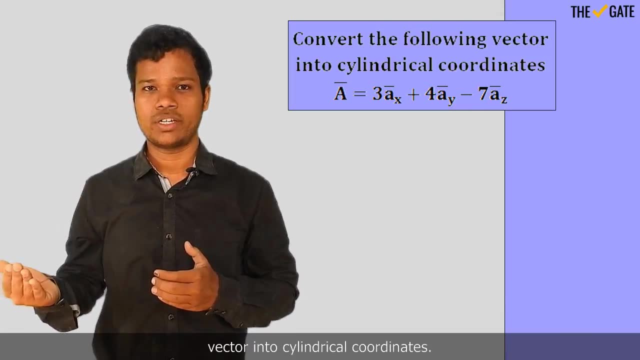 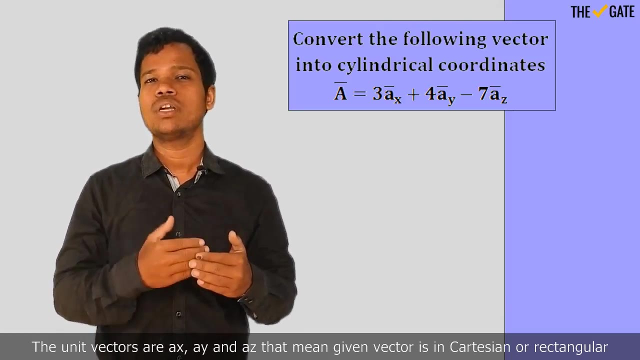 In the question. the given vector is 3AX plus 4AY minus 7AZ and we want to represent this vector into cylindrical coordinates. Now you can easily see from the question. the given vector is in Cartesian coordinate system. The unit vectors are AX, AY and AZ. 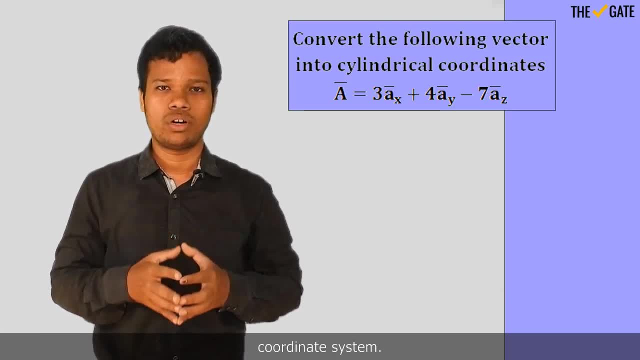 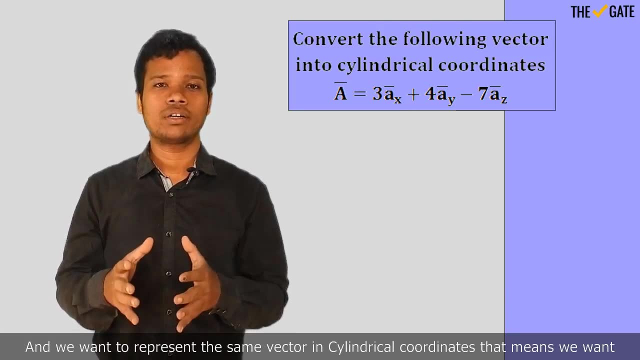 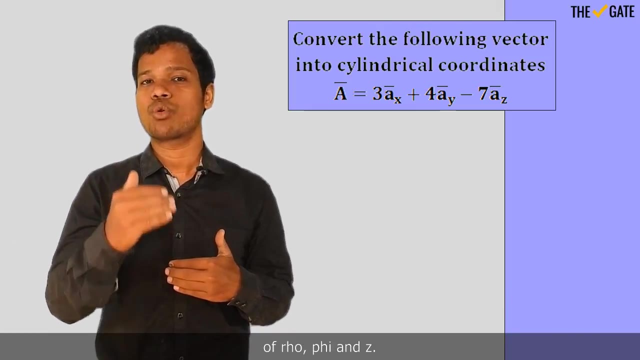 That means given vector is in Cartesian or rectangular coordinate system and we want to represent the same vector into cylindrical coordinates. That means we want row component, phi component and Z component and we want to represent the vector in terms of row, phi and Z. 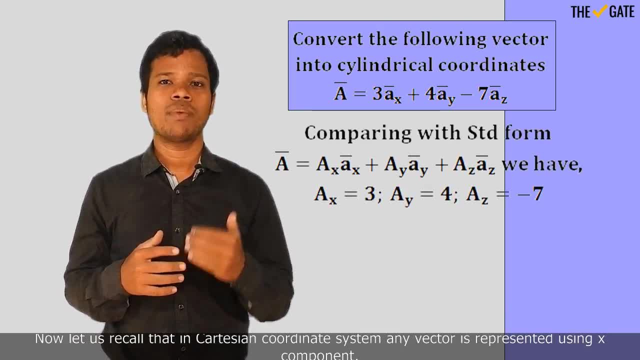 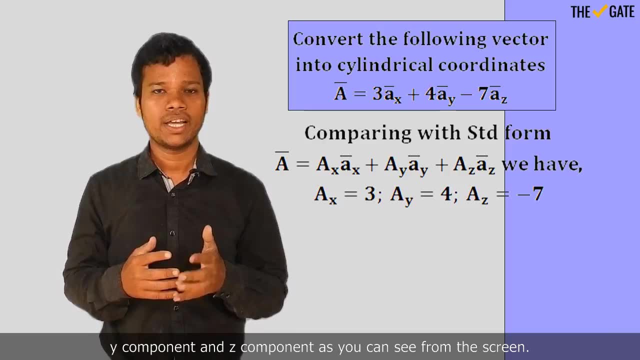 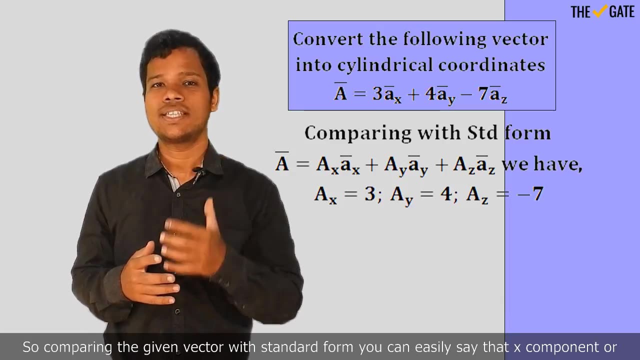 Now let us recall that in Cartesian coordinate system, any vector is represented using X component, Y component and Z component, as you can see from the screen. So, comparing the given vector with the standard form, you can easily say that X component is a component or capital. AX will be equal to 3.. 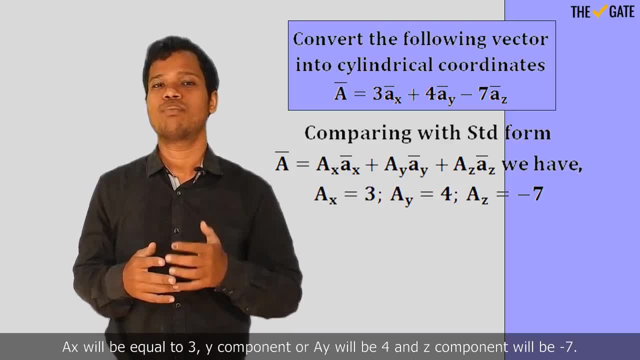 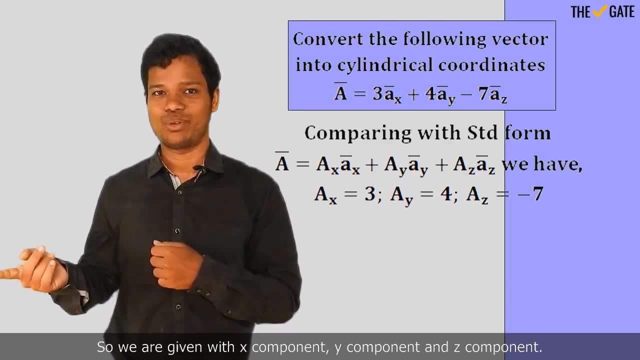 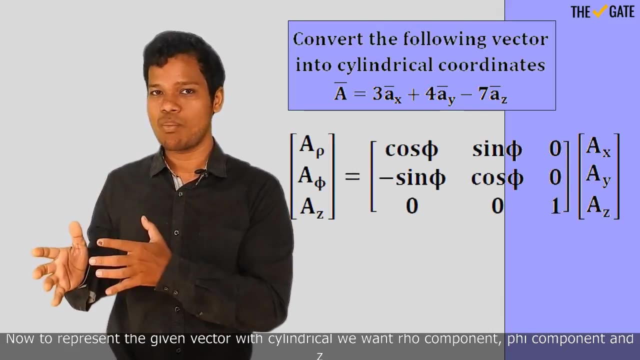 Y component or capital AY equal to 4 and Z component will be minus 7.. So we are given with X component, Y component and Z component. Now to represent the given vector into cylindrical, we want row component, phi component and Z component. 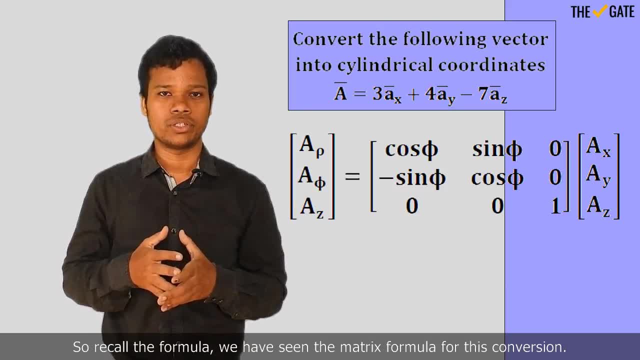 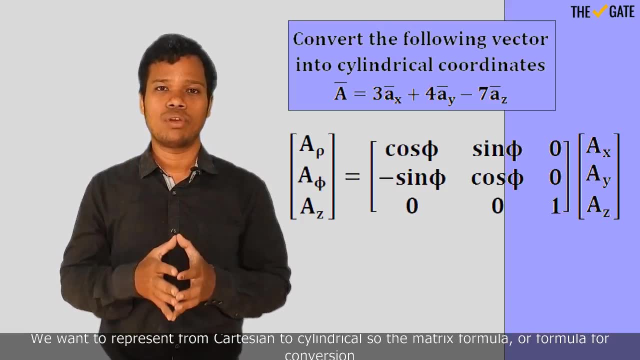 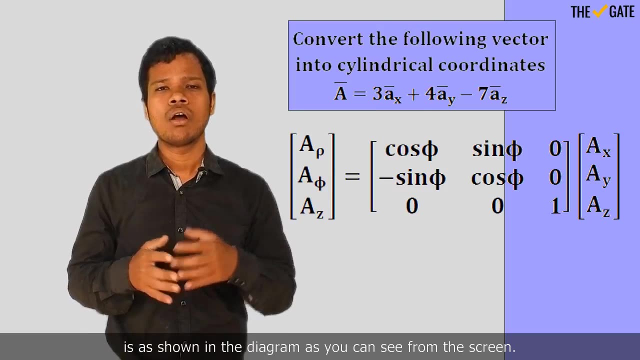 So recall the formula. we have seen the matrix formula for this conversion. We want to represent cartesian to cylindrical. so the matrix formula or formula for conversion is as shown in the diagram. you can easily see from the screen putting the values of capital, ax, capital ay and capital. 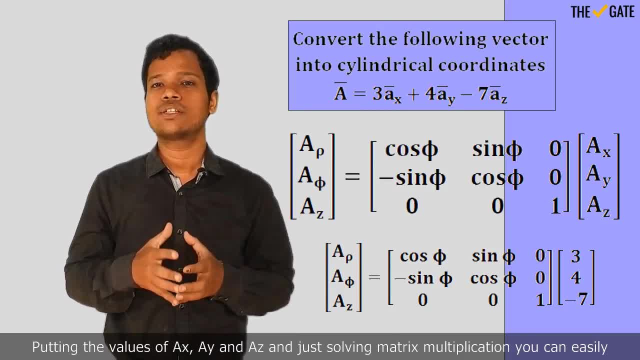 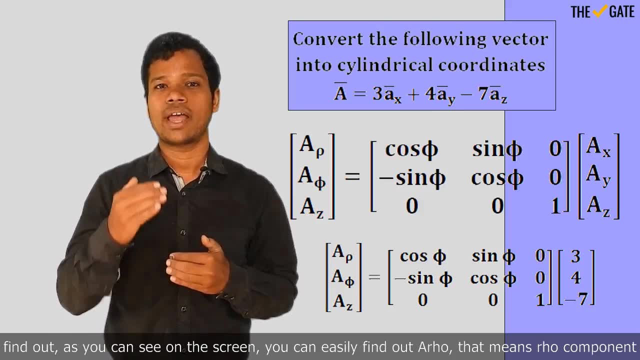 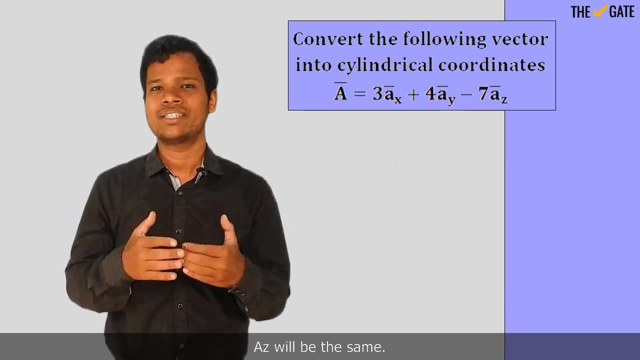 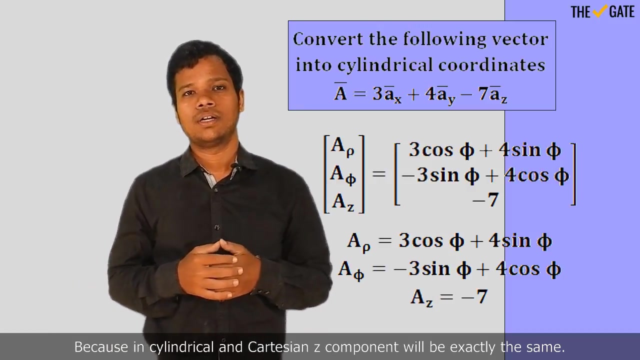 z and just solving matrix multiplication you can easily find out. as you can see on the screen, you can easily find out: capital a rho- that means rho component. capital a phi- that means phi component, and capitalized- capitalized. it will be the same because in cylindrical and cartesian z component is exactly the same. so this is how we can represent vector: from cartesian to cylindrical. 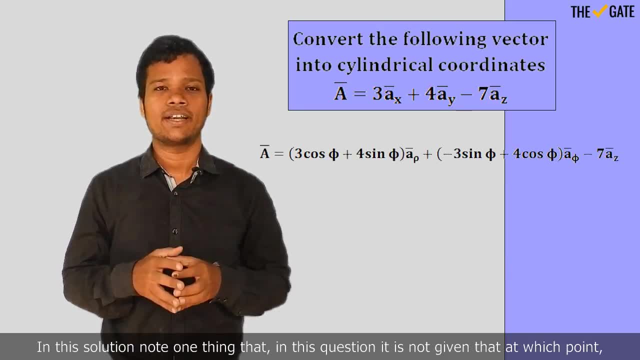 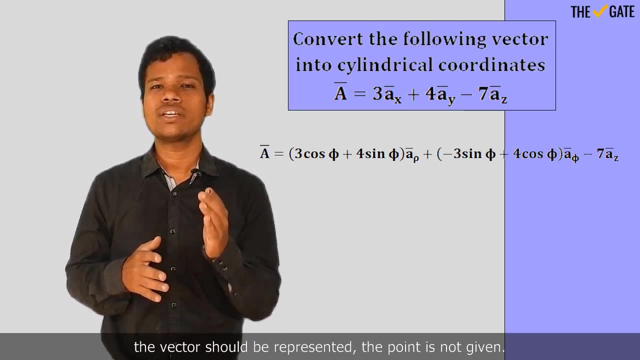 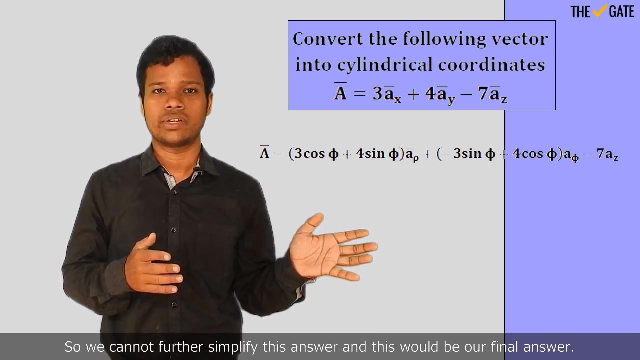 in this solution. note one thing: that in this question it is not given that at which point the vector should be represented. the point is not given. that means we cannot calculate phi. and as we cannot calculate phi, as we are not given with phi, we cannot calculate sin phi and cos phi. so we cannot further simplify this answer. 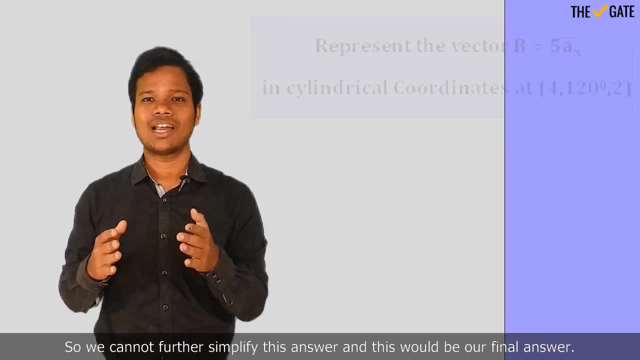 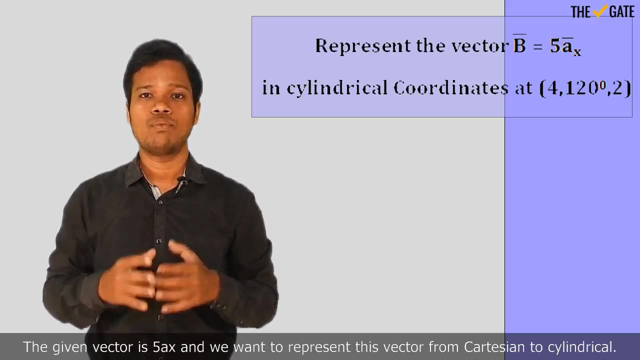 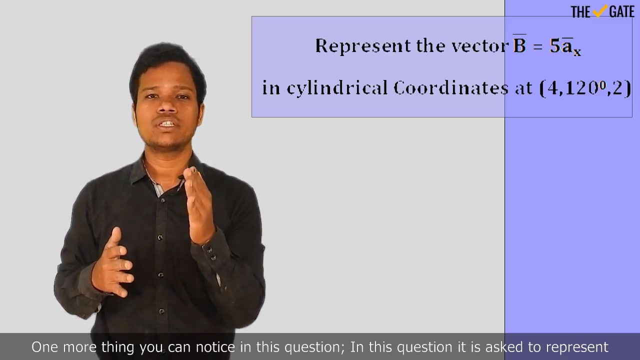 and this would be our final answer. let us take next question. as you can read from your screen, the given vector is phi u ax and we want to represent this vector from Cartesian to cylindrical. one more thing you can notice in this question: in this question it is asked to represent the vector at certain point. 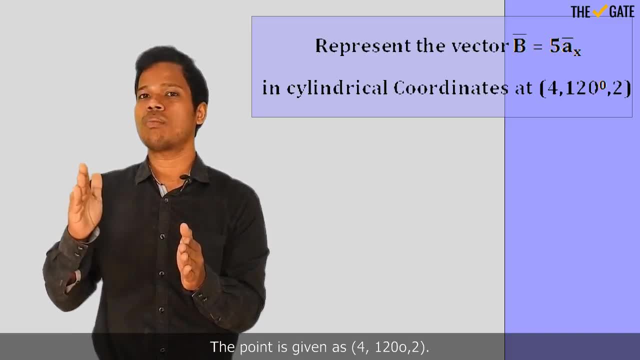 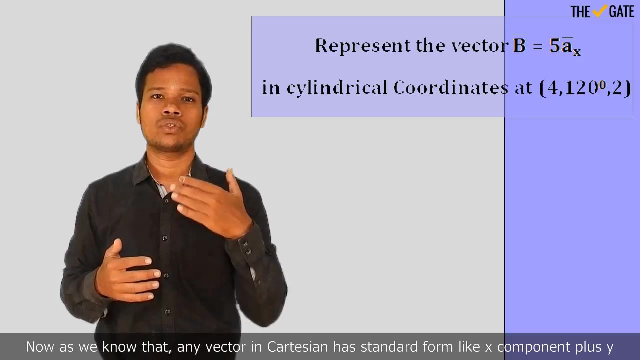 the point is given as 4 comma 120 degree comma 2, so we will think about later. first of all, let us convert the given vector into cylindrical. the given vector is in Cartesian. now, as we know that any vector in Cartesian has standard form like x component plus Y component plus Z component. so, comparing with the 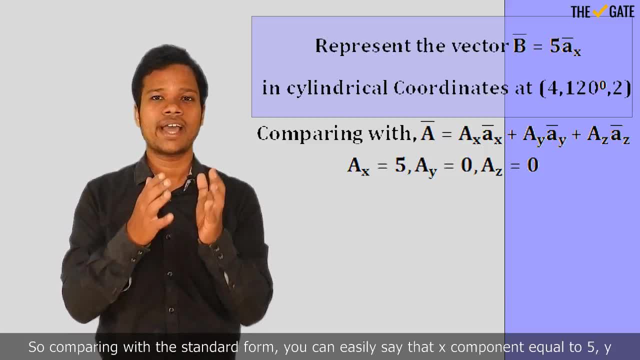 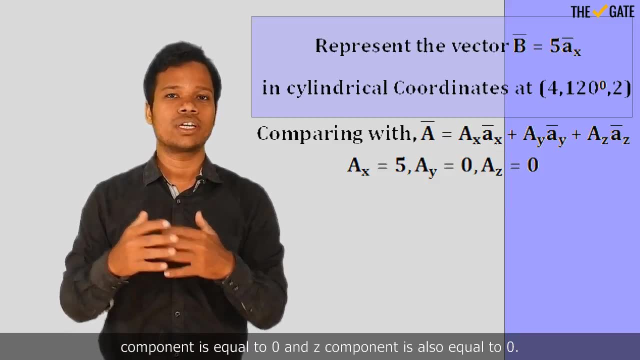 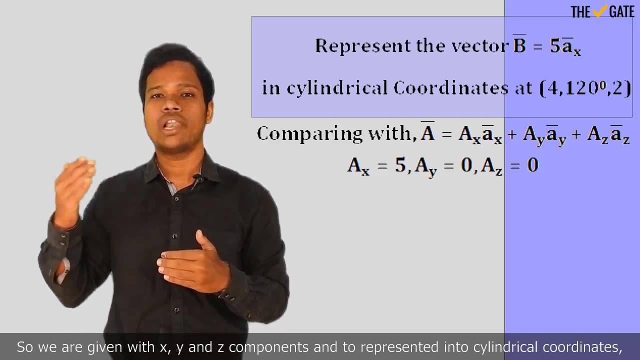 standard form you can easily say that X component equal to Phi u, Y component equal to zero and Z component is also equal to zero. so we are given with x, Y and Z components and now to represent into cylindrical coordinates we want go Phi and Z components. so once again, recall the relevant formula, as we have. 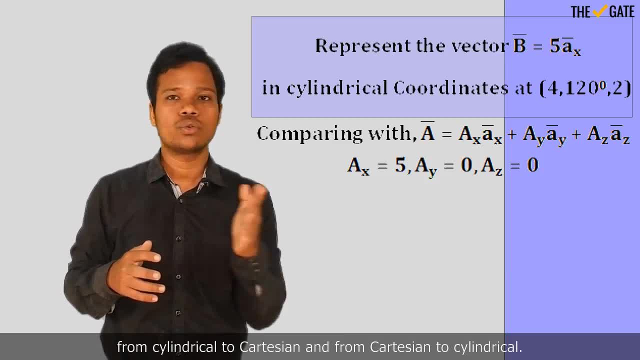 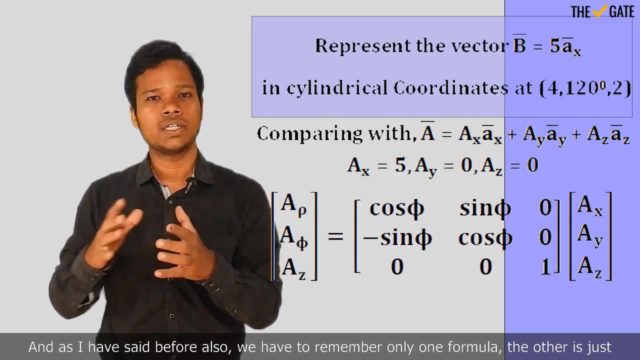 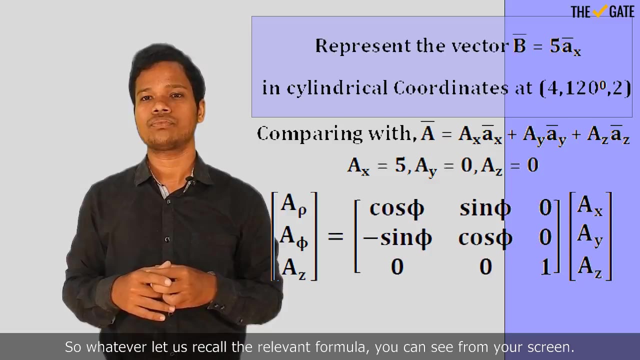 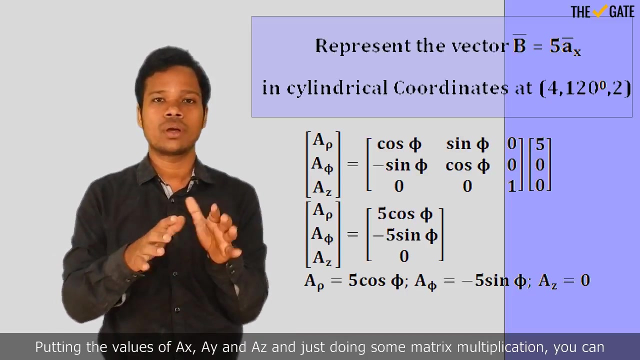 seen. we have seen two formulae, from cylindrical to cartesian and from cartesian to cylindrical, and, as i said before, also, you have to remember only one formula. the other is just only the transpose. so, whatever, let us recall the relevant formula you can see from your screen putting the values of capital ax, capital ay and capital z and just doing some matrix multiplication. 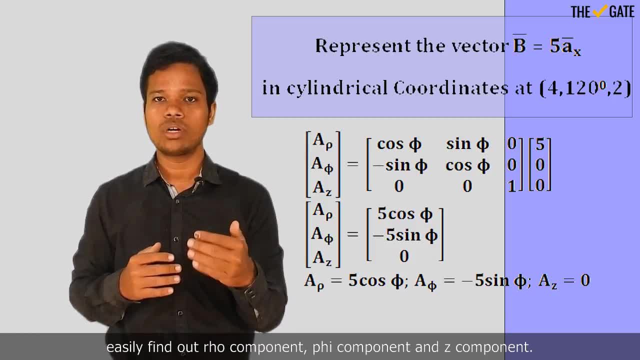 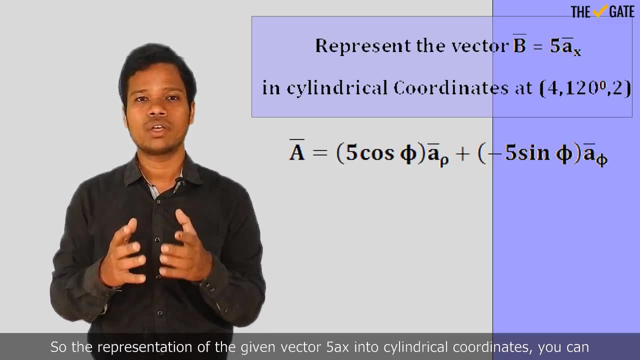 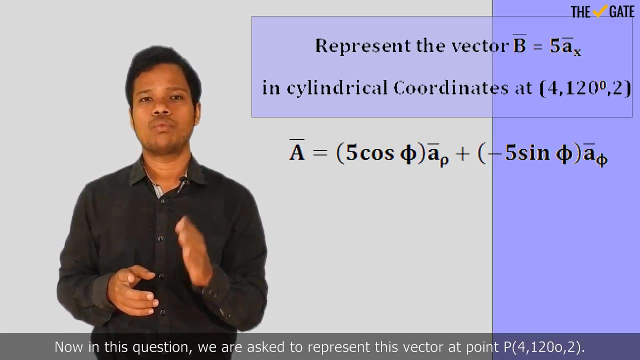 you can easily find out rho component, phi component and z component. so the representation of the given vector 5 ax into cylindrical coordinates you can see from your screen. now in this question we are asked to represent this vector at point p, 4 comma, 120 degree comma 2. 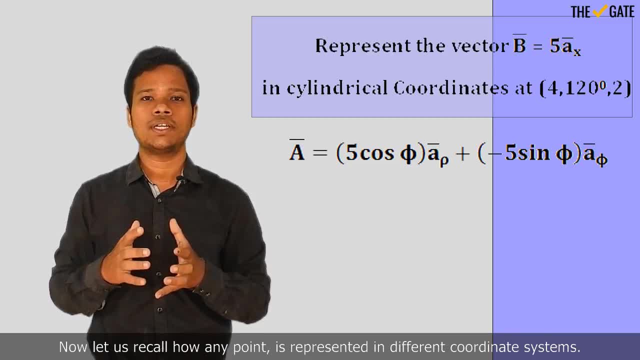 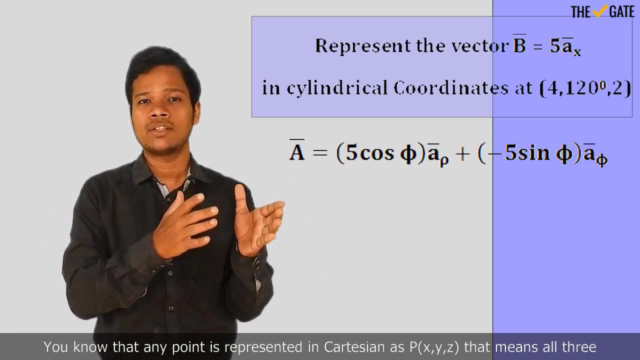 now let us recall how any point is represented in this vector: p 4, comma 120 degree, comma 2, in different coordinate systems. You know that any point is represented in Cartesian as P, X, Y, Z. that means all three are numbers. 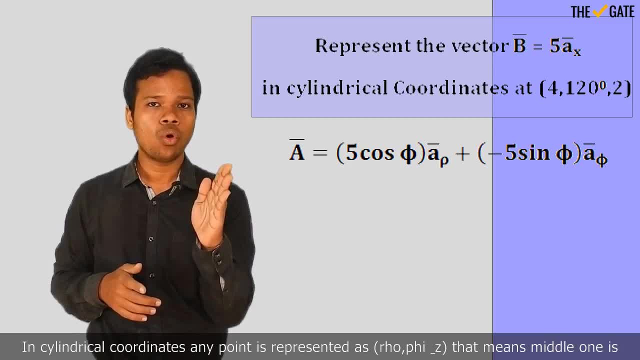 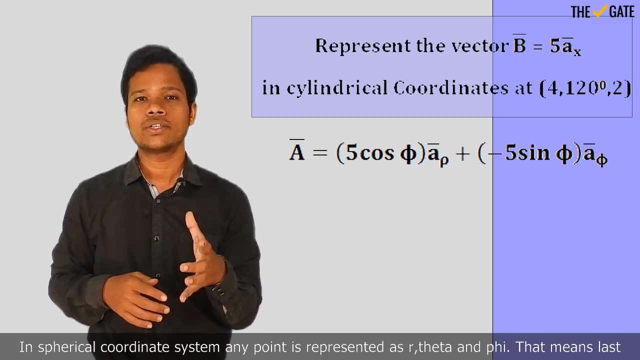 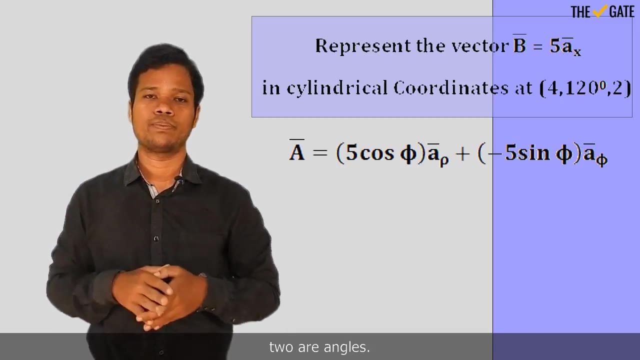 In cylindrical coordinates any point is represented as rho, phi and z. that means middle one, is the angle. In spherical coordinate system any point is represented as r, theta and phi. that means last two are angles. So what I'm trying to say you in the given question, 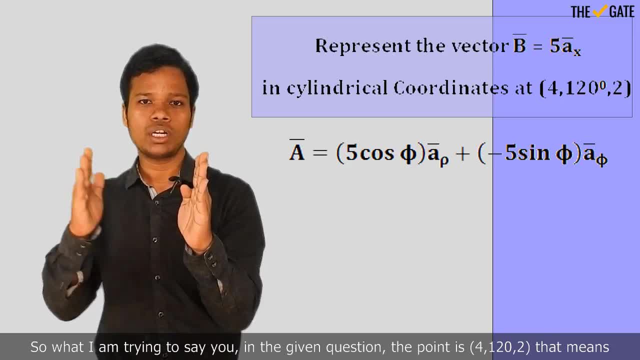 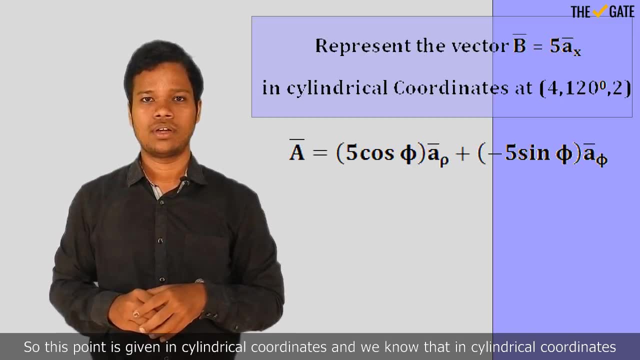 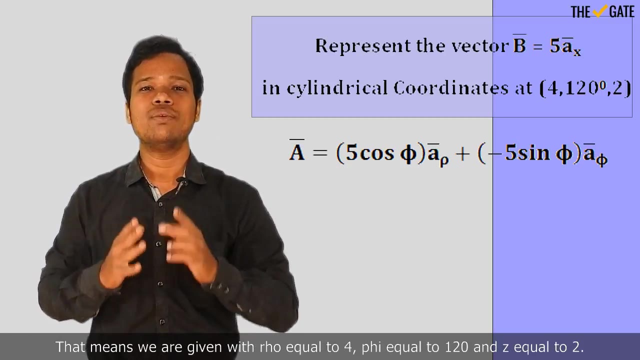 the point is four comma 120 degree. comma two, that means middle one is the angle. So this point is given in cylindrical coordinates And we know that in cylindrical coordinates any point is rho, phi and z. That means we are given with rho equal to four. 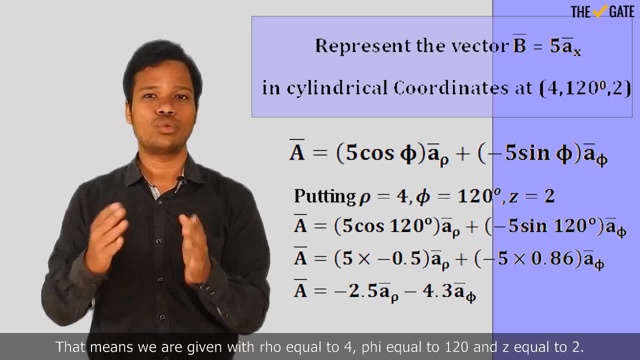 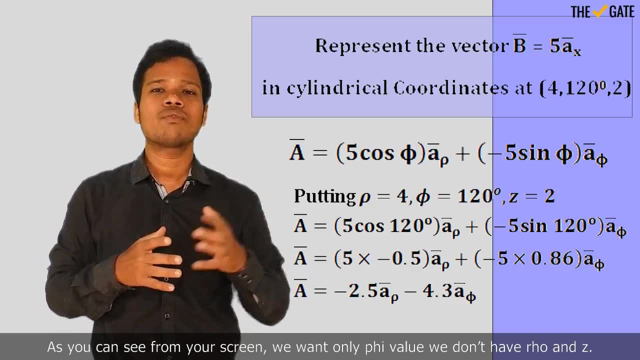 phi equal to 120, and z equal to two. So putting these values of rho, phi and z into our last step, we can conclude to the answer. As you can see from your screen, we want only phi value. We don't have rho and z. 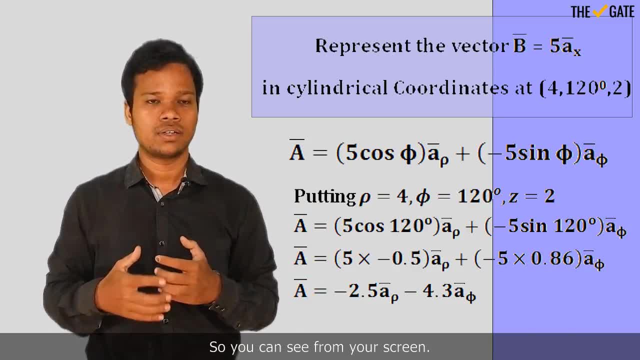 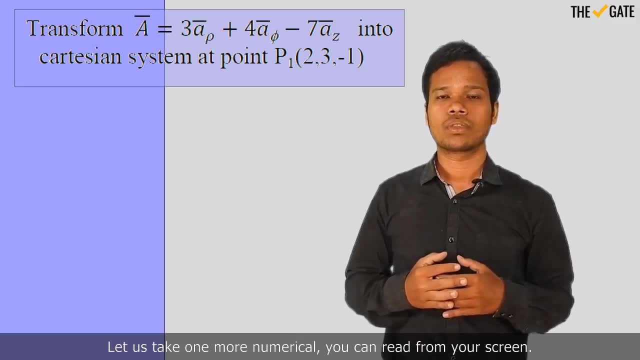 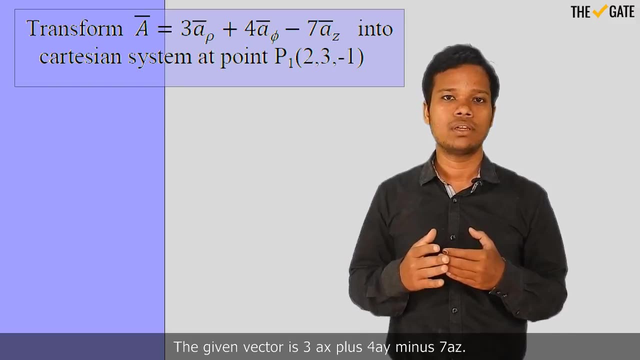 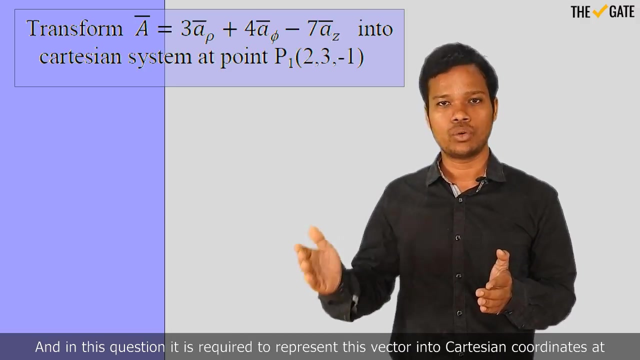 So putting the phi. you can conclude to final answer, as you can see from your screen. Let us take one more numerical. you can read from your screen: The given vector is three A rho plus four A phi, minus seven A z and in this question it is required to represent this vector. 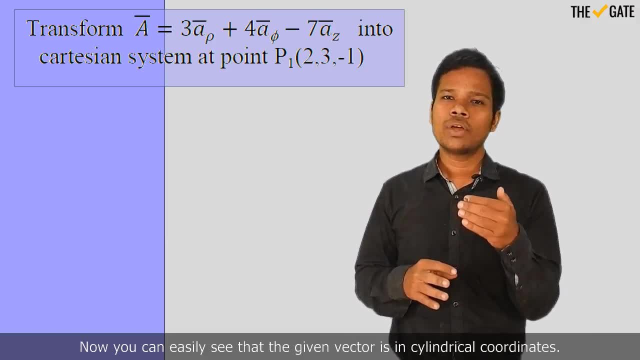 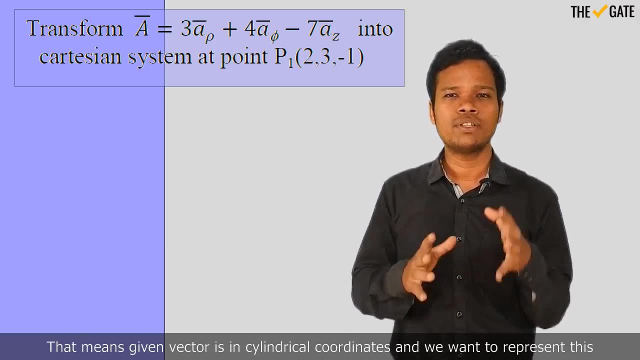 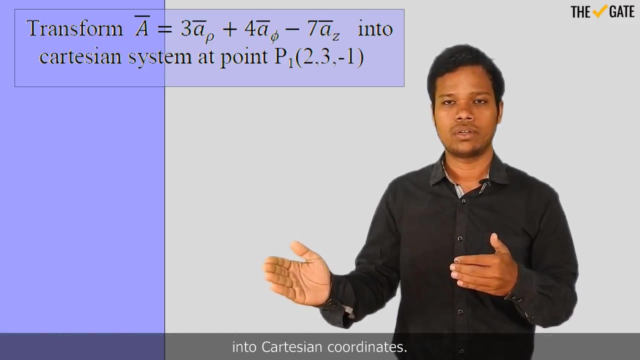 at certain point. now you can easily say that the given vector is in cylindrical coordinates. it has unit vectors a, rho, a, phi, a, z. that means given vector is in cylindrical coordinates and we want to represent this into cartesian coordinates. now we already know that any vector in cylindrical coordinate has 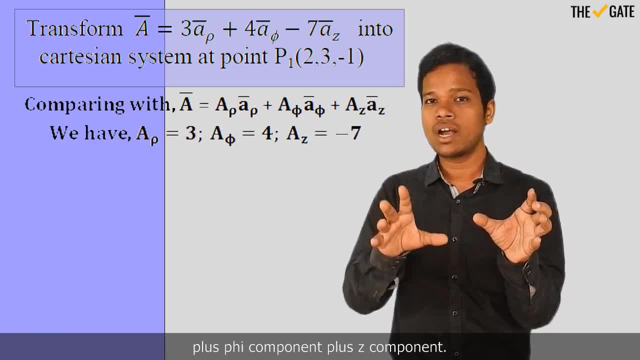 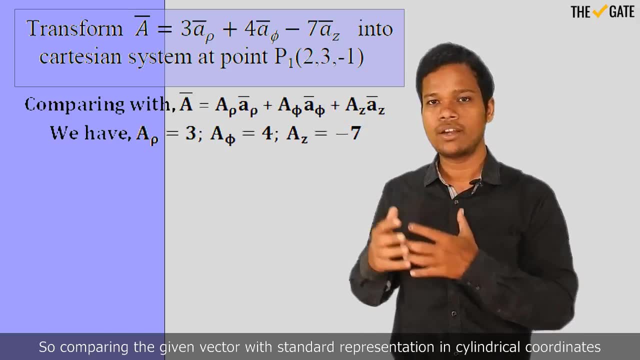 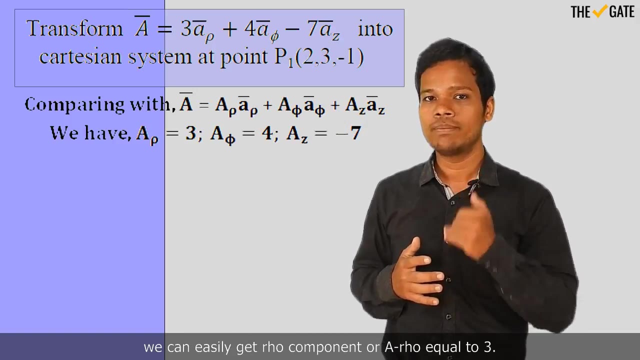 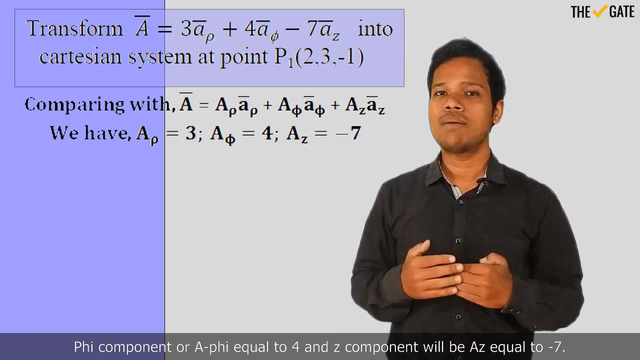 standard form like rho component plus phi component plus z component. so comparing the given vector with standard representation in cylindrical coordinates, we can easily get rho component or capital. a rho equal to 3, phi component or capital. a phi equal to 4 and z component will be a z equal to minus 7.. 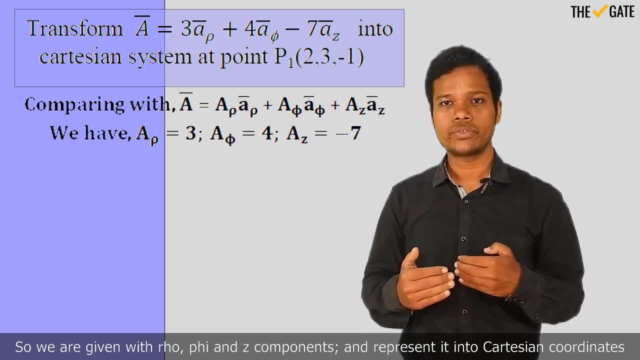 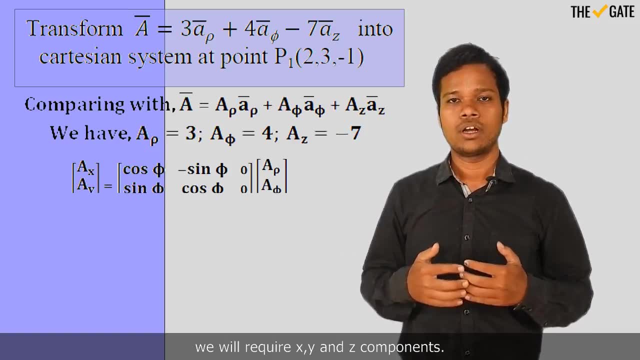 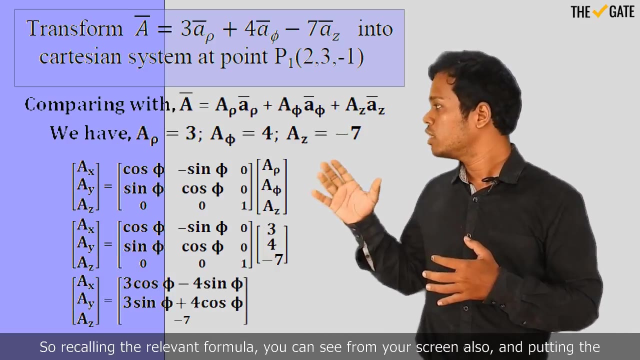 so we are given with rho, phi and z components and to represent it into cartesian coordinates we will require x, y and z components. so recalling the relevant formula- you can see from your screen also- and putting the values for rho, phi and z components and doing simple matrix. 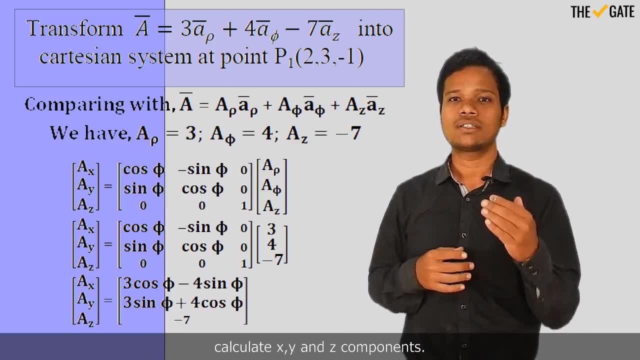 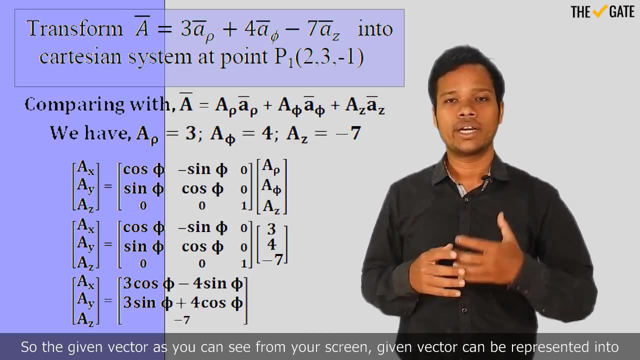 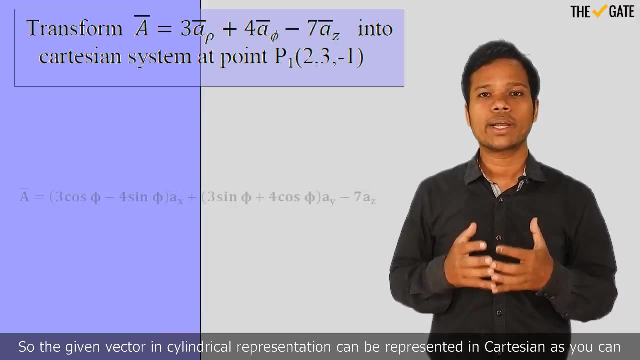 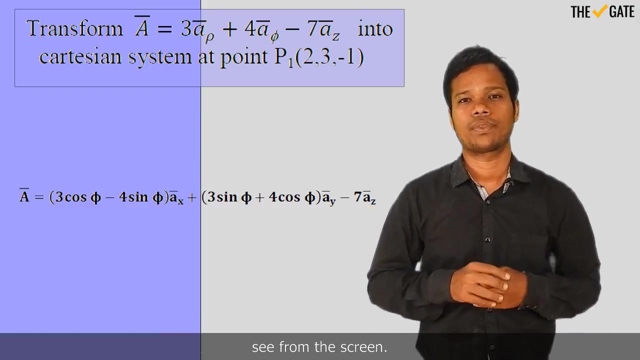 multiplication. we can easily calculate x, y and z components, as you can see from your screen. given vector can be represented into cartesian coordinates, as you see. so the given vector in cylindrical representation can be represented in cartesian, as you can see on the screen. now, my dear, you can notice one thing over here. 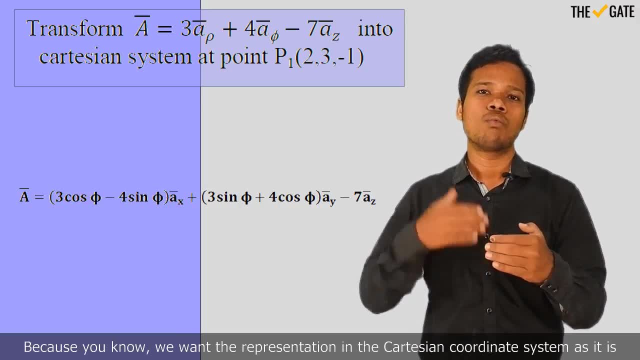 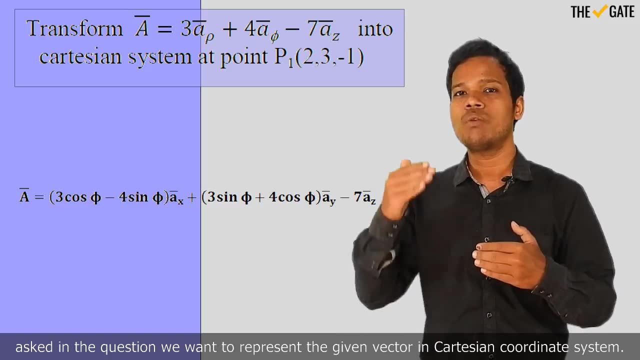 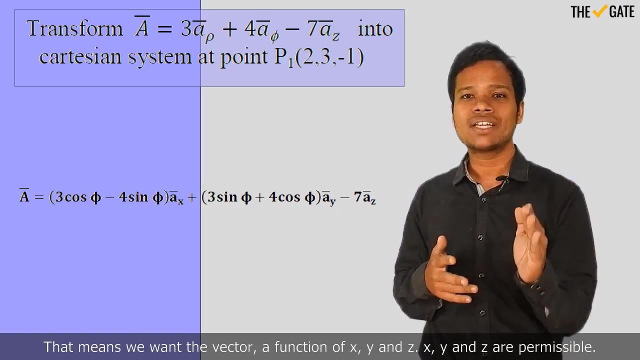 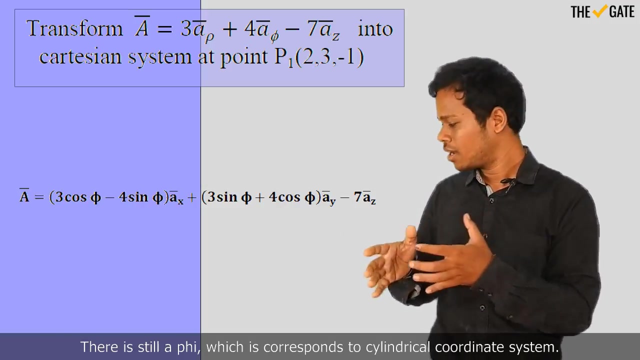 this could not be our final answer because you know we want the representation in cartesian coordinate system. we want to represent the given vector in cartesian coordinate system. that means we want the vector a function of x, y and z. x, y and z are permissible. but what you can see in our answer there is still. 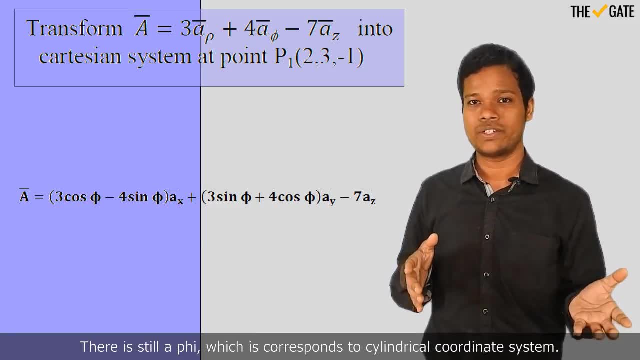 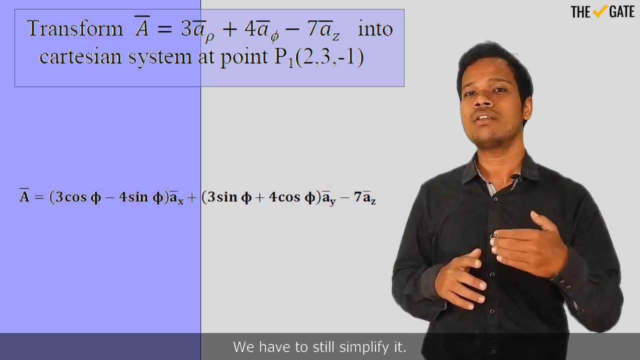 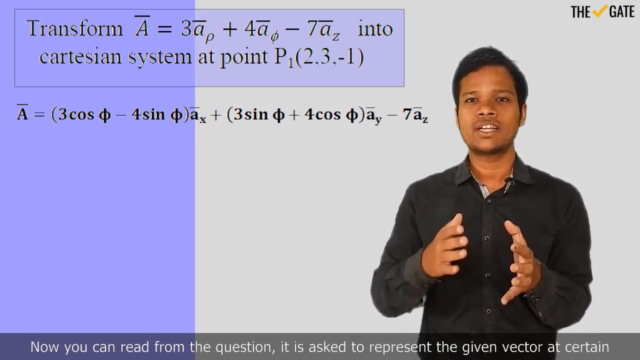 a phi, which is, corresponds to cylindrical coordinate system. so what i am trying to say you. this could not be our final answer. we have to still simplify it now. you can read from the question. it is asked to represent the given vector at certain point. the point is given as: 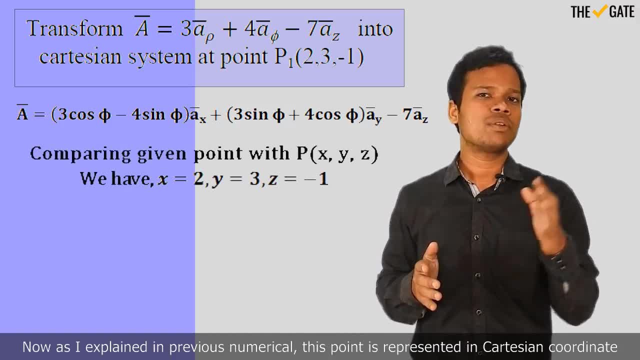 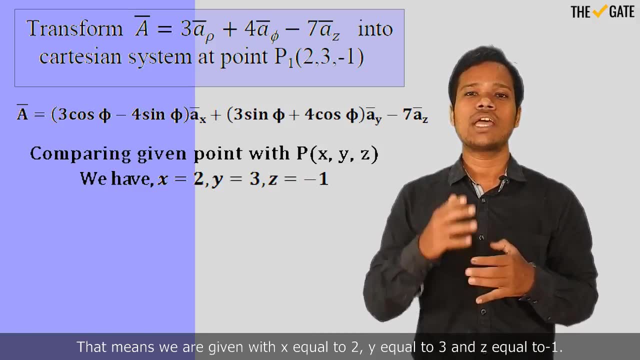 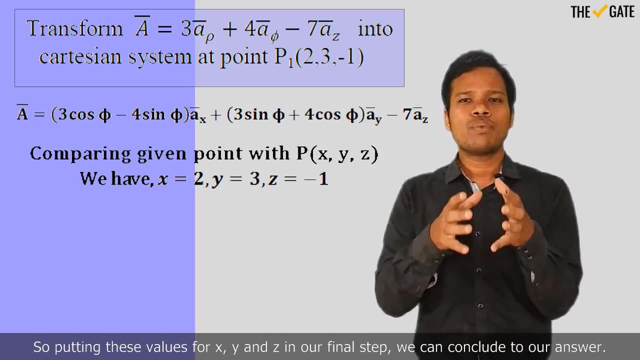 2, 3 minus 1. now, as i explained in previous numerical, this point is represented in cartesian coordinate system. that means we are given with x equal to 2, y equal to 3 and z equal to minus 1. so putting these values for x, y and z. 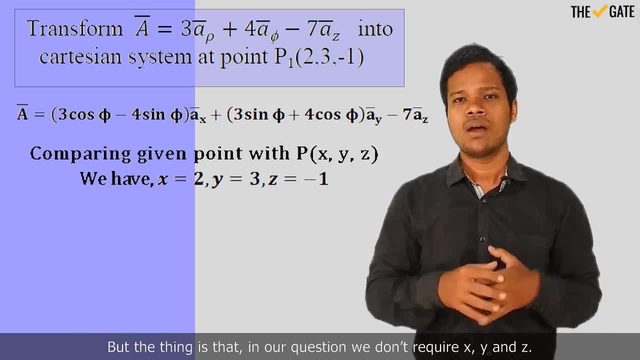 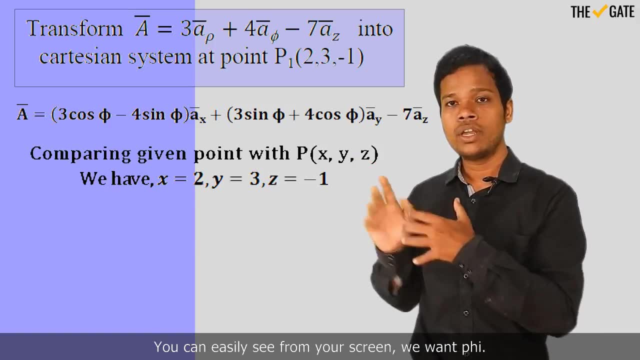 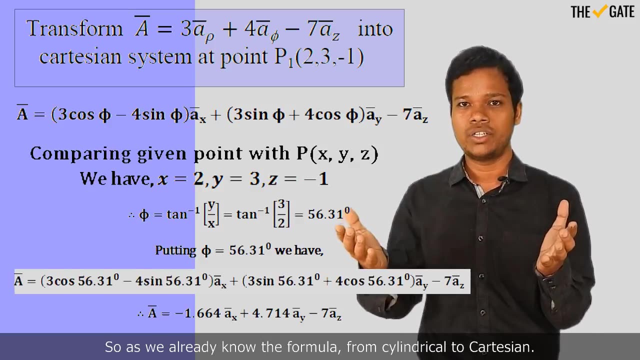 into our final step, we can conclude to our answer. but the thing is that in our question we don't require x, y and z. you can easily see from your, from your screen, we want phi. so, as we already know, the formula, from cylindrical to cartesian phi can be easily calculated using the formula. 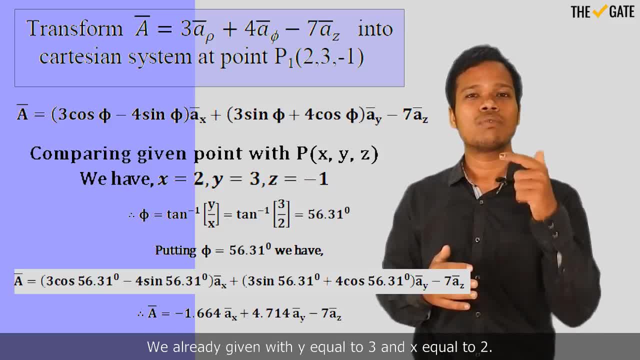 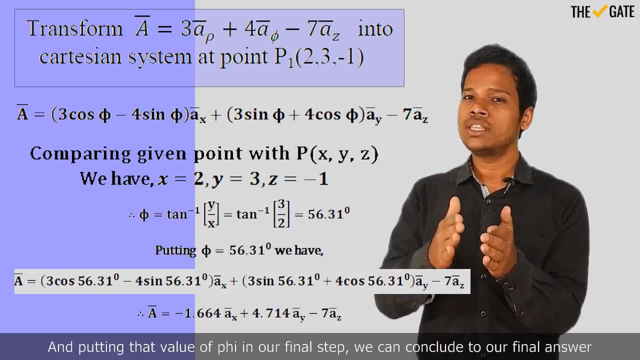 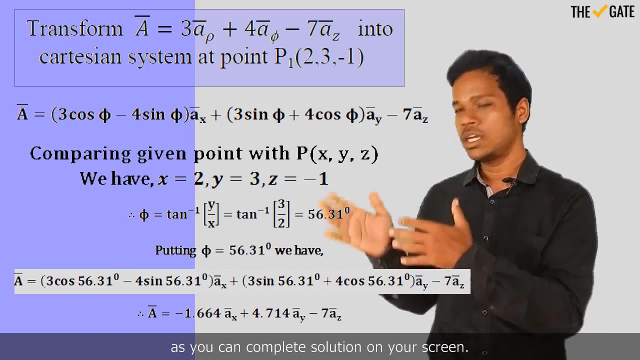 tan inverse y by x we already given, with y equal to 3 and x equal to 2. so first of all we can calculate phi and putting that value of phi in our final step, we can conclude to our answer, as you can see complete solution on your screen.